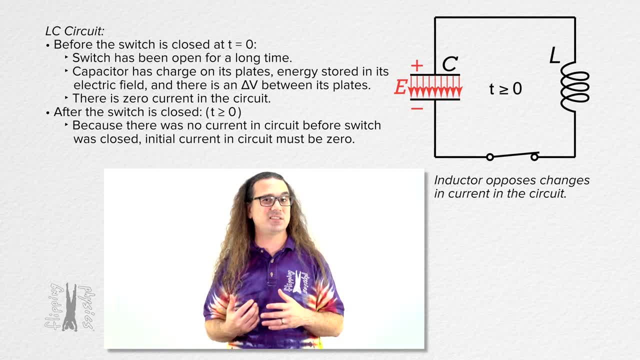 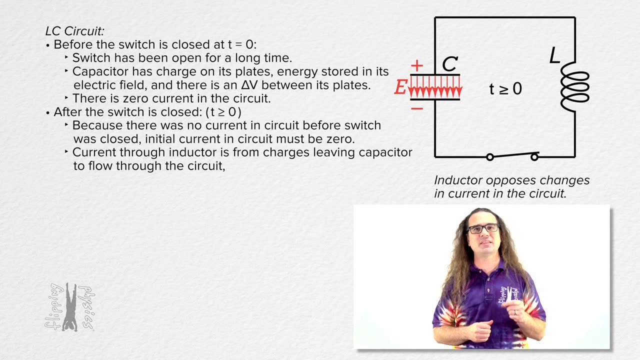 Billy…. An inductor-capacitor circuit does not reach a steady-state current like an inductor-resistor circuit. But then what happens? We are about to figure that out, Great. The current passing through the inductor is caused by charges leaving the capacitor. Therefore. 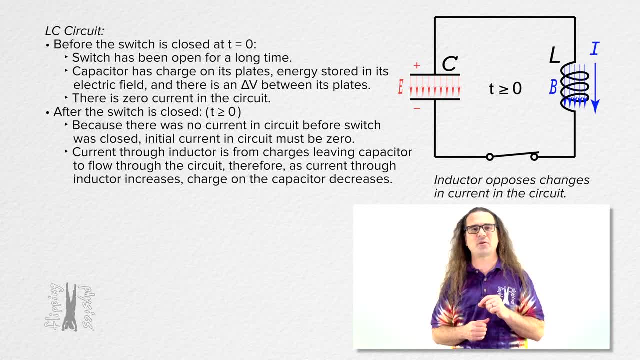 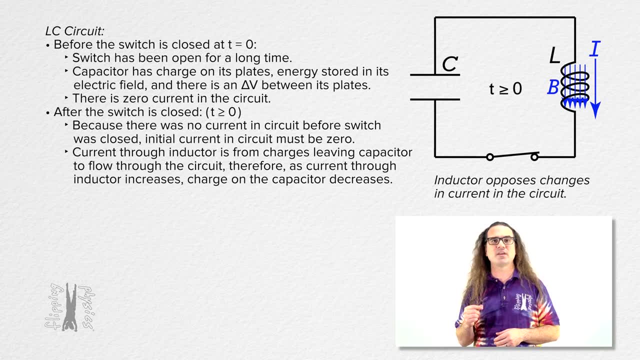 as current through the inductor increases, charge on the capacitor decreases. The current moving through the inductor causes a magnetic field in the inductor. Therefore, as the current passing through the inductor increases, charge on the capacitor decreases. As the magnitude of the electric field in the capacitor decreases. 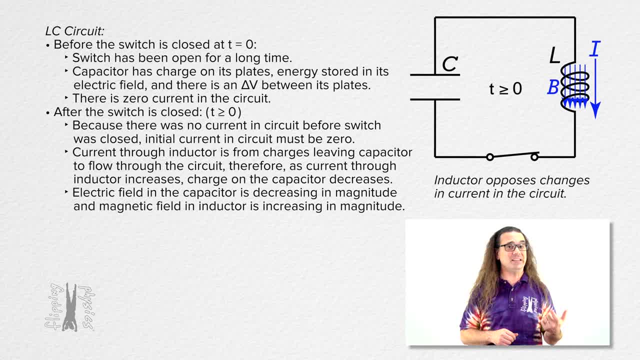 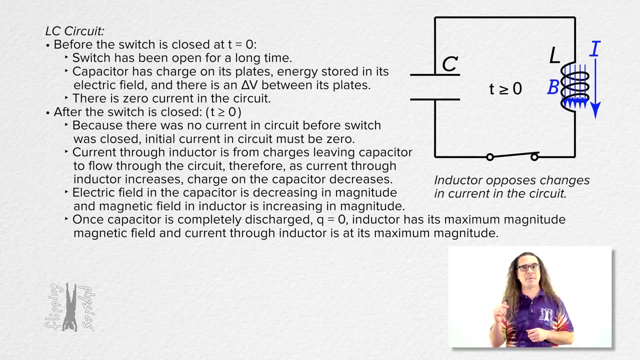 the magnitude of the magnetic field in the inductor increases Once the charge on the capacitor is completely discharged. the charge on the plates of the capacitor equals zero. the inductor has its maximum magnitude magnetic field and the current through the inductor is at its maximum magnitude. Current continues to flow and builds up charges. 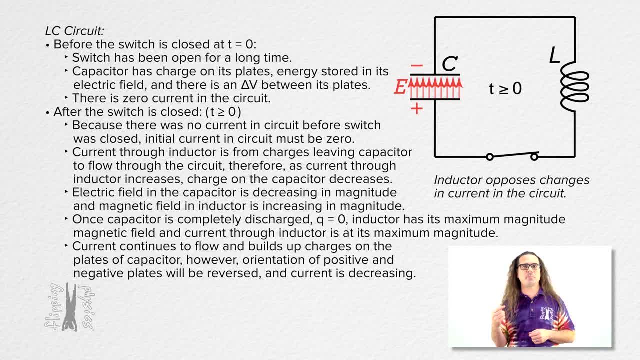 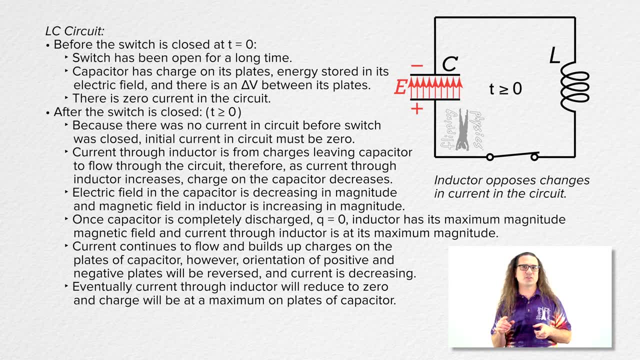 on the plates of the capacitor. However, the orientation of the positive and negative plates will be reversed and the current is decreasing. Eventually, the current through the inductor will reduce to zero and charge will be at a maximum on the plates of the capacitor. 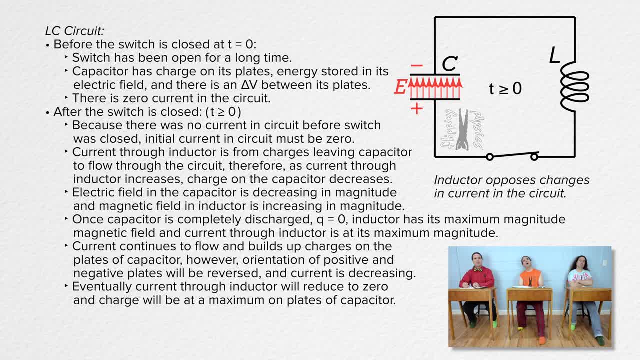 But the charges on the plates of the capacitor are reversed from where they were when the switch was closed, right, Correct. Does that mean the whole process repeats itself, only in reverse this time? Yes, it does. It's simple, harmonic motion. 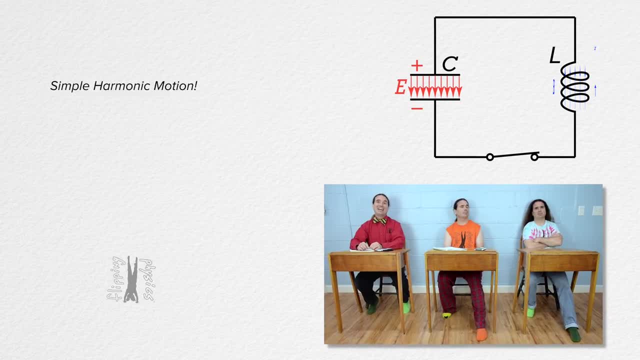 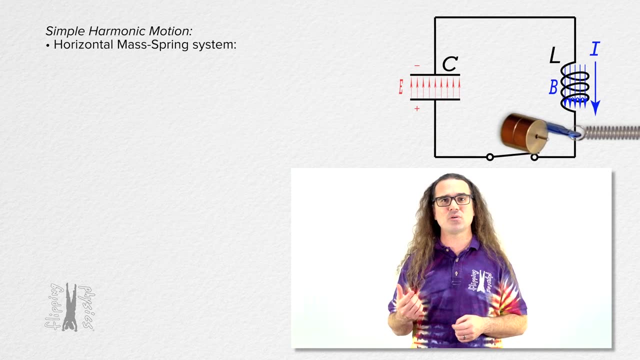 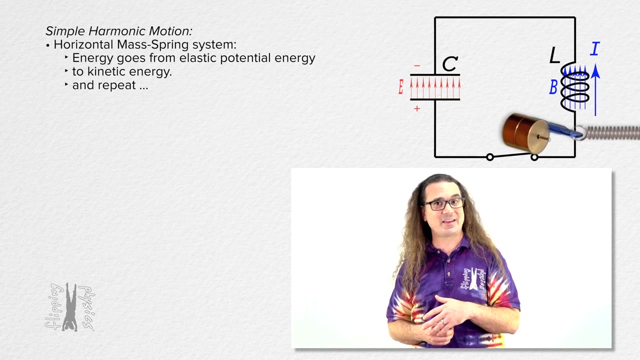 Simple, harmonic motion. It does not look like. it Looks simple. A horizontal mass-spring system is a good analogous situation. As the mass oscillates back and forth, the mechanical energy goes from being elastic potential energy to kinetic energy, to elastic potential energy to kinetic energy. 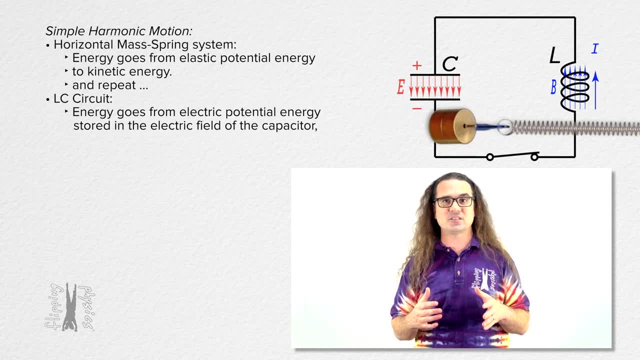 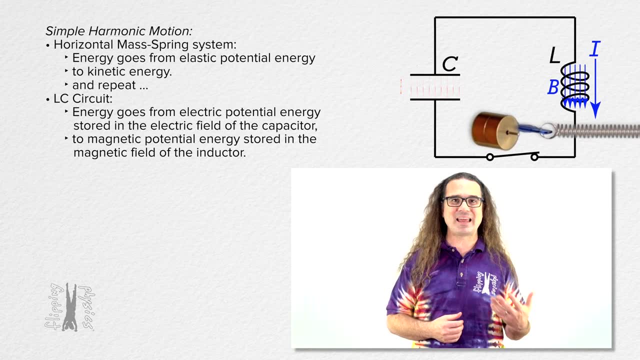 Just like in the inductor-capacitor circuit, the energy in the system goes from being electric potential energy stored in the electric field of the capacitor to magnetic potential energy stored in the magnetic field of the inductor, to energy in the capacitor, to energy in the inductor. 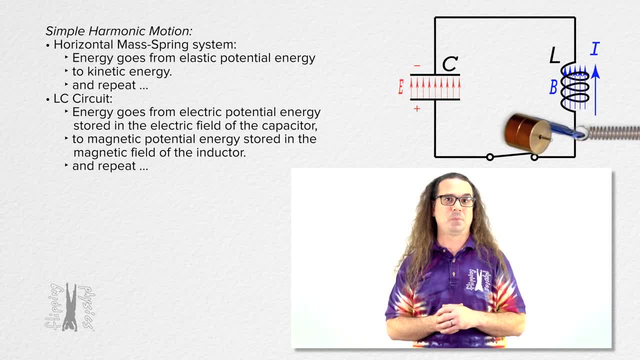 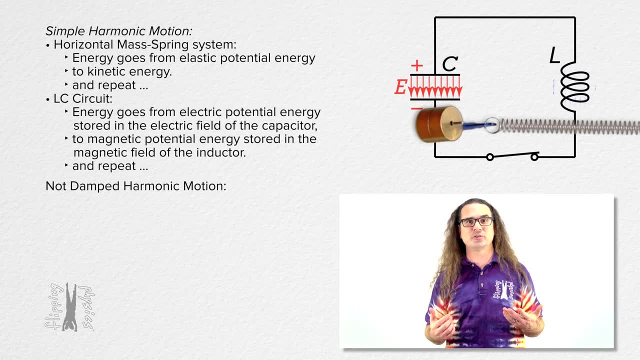 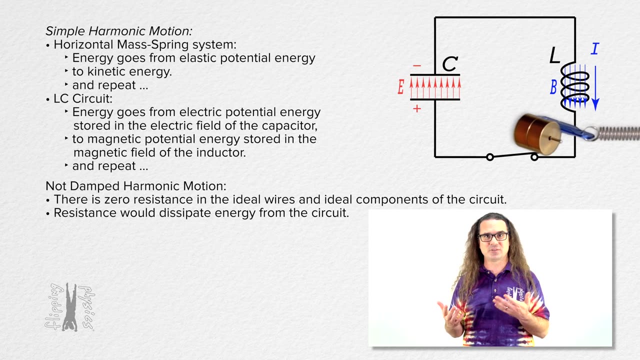 They are both examples of simple harmonic motion. I still don't think it looks simple. Yeah Well, it's not damped harmonic motion because there is zero resistance in the wires of this LC circuit. Resistance in the circuit would dissipate energy from the circuit. 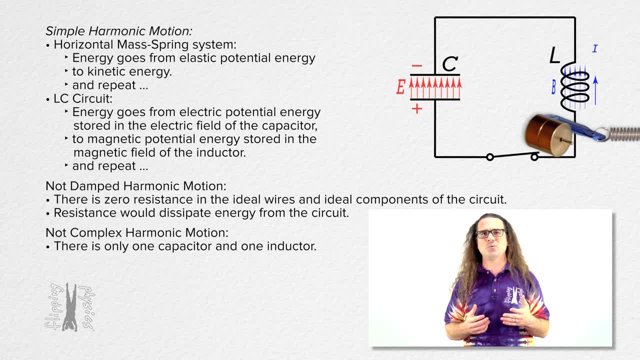 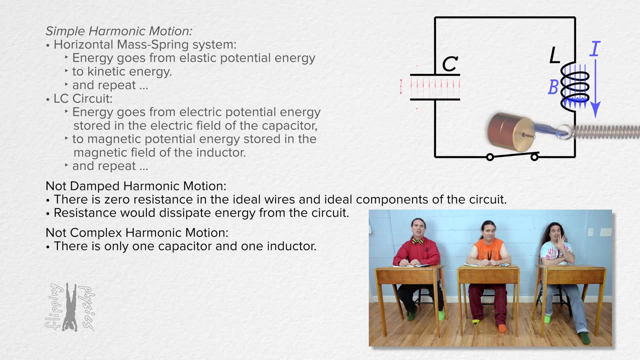 And it's not complex harmonic motion, because there is only one capacitor and one inductor and not some complicated combination of multiple inductors, capacitors and resistors. So yeah, an ideal LC circuit is simple, harmonic motion. Okay, Yeah, I got it, Thanks. 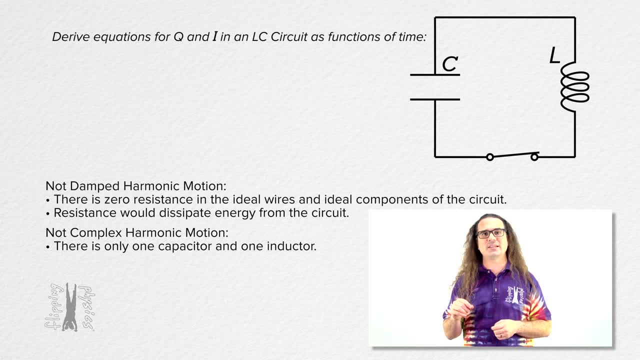 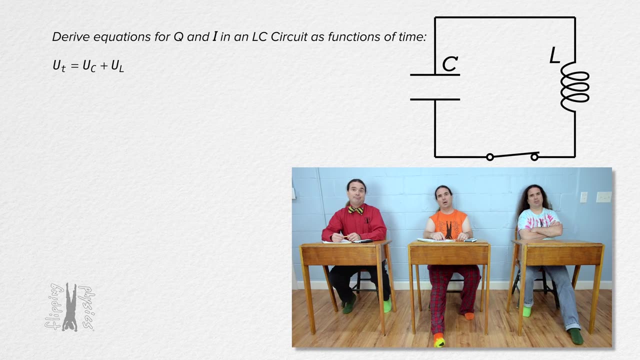 Okay, Let's derive equations for charge on the plates of the capacitor and current through the inductor as functions of time. To do that, let's start with an equation for the total potential energy in the circuit Bo, please. Okay, The total potential energy in the circuit equals the electric potential energy in the. 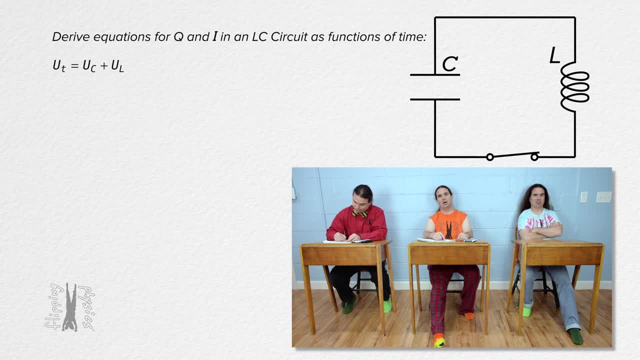 capacitor plus the magnetic potential energy in the inductor, The electric potential energy stored in the capacitor equals …. Well, we have three equations for that. Which one do you want me to use? Please use charge squared divided by 2 times capacitance. 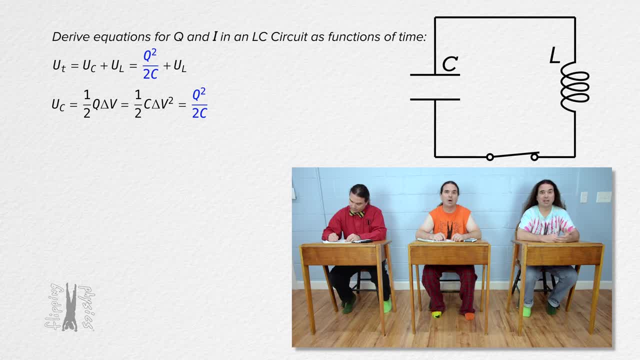 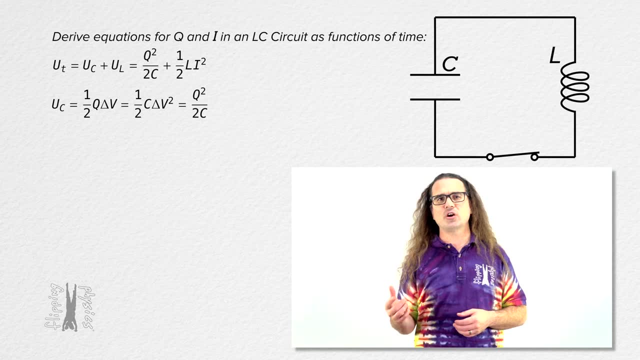 Sure, We can use that one. And the energy stored in an inductor equals one-half inductance times, current squared In an inductor-capacitor circuit charge and current are changing as functions of time, So we can use the electric potential energy stored in the capacitor. 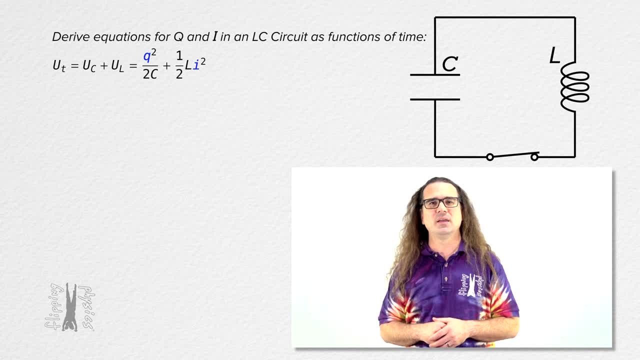 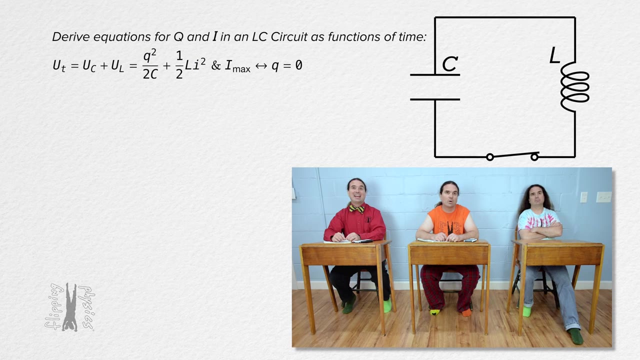 Let's use lowercase variables for q and i. Typically, we use uppercase symbols for constants and lowercase symbols for variables. Also, we already discussed this. however, let's specifically identify that current through the inductor is at its maximum magnitude when charge to the capacitor equals zero And charge to the capacitor is at its maximum when the current 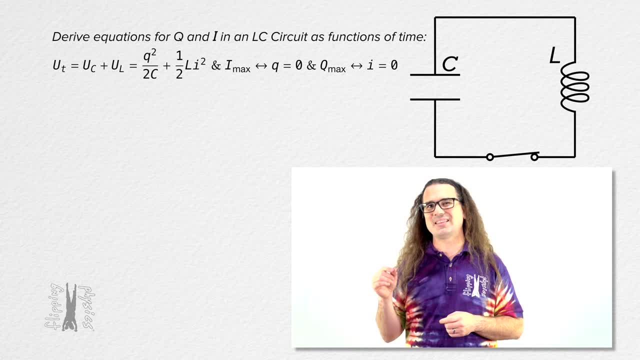 through the inductor is zero. Next, let's take the derivative of the total energy equation with respect to time. Let's take the derivative of the total energy equation with respect to time. Bobby, what is the derivative of the total energy of the LC circuit with respect to time equal to? 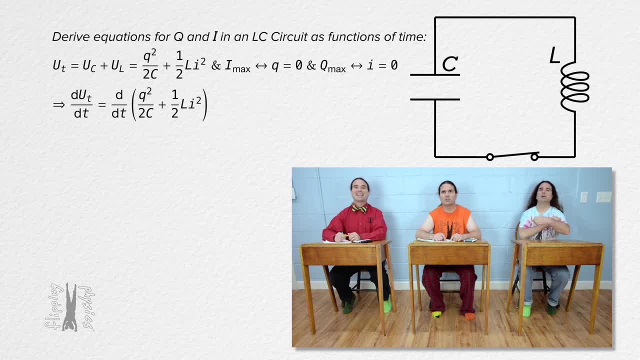 The derivative of total energy with respect to time equals …. Well, this circuit is an ideal circuit with zero resistance, so zero energy is being dissipated from the circuit. That means the total energy in the circuit does not change over time. so the time rate of change in the circuit 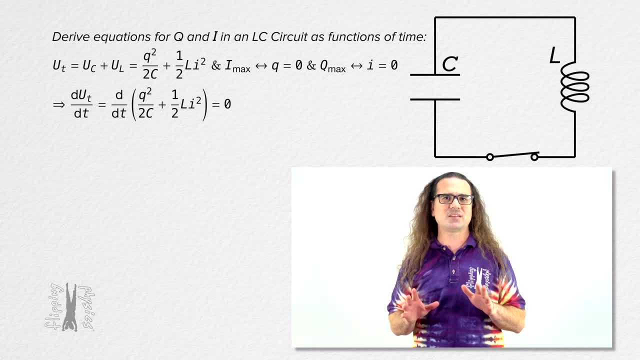 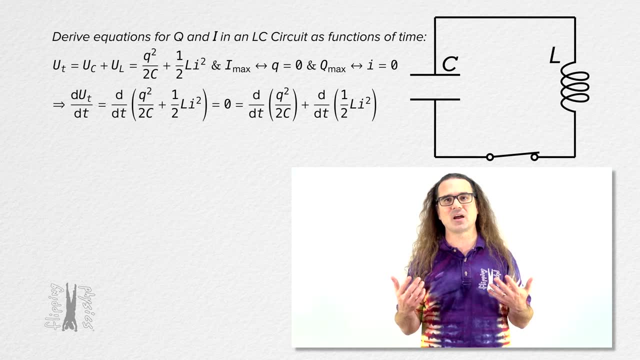 equals zero, Correct? And just to make the next question a little bit easier, let's take the derivative of the total energy equation with respect to time And just to make the next step clear, realize we can take the derivative of each energy expression independently, because they are added together in our equation. 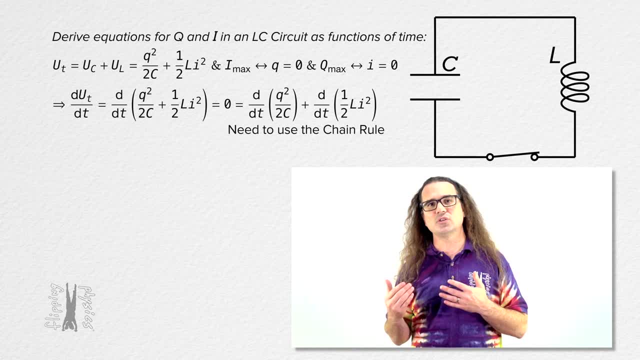 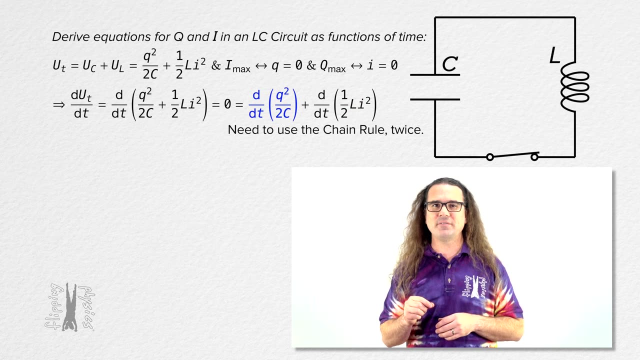 Now, in order to take these derivatives, we need to use the chain rule twice, Because the variables for charge and current both change with respect to time. however, the variable t is not in either of those equations. In other words, the derivative with respect to time of charge squared divided by: 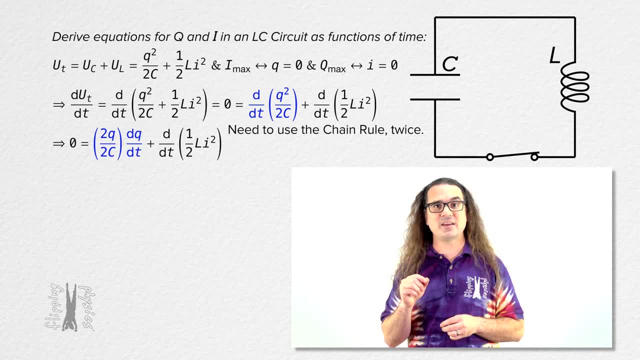 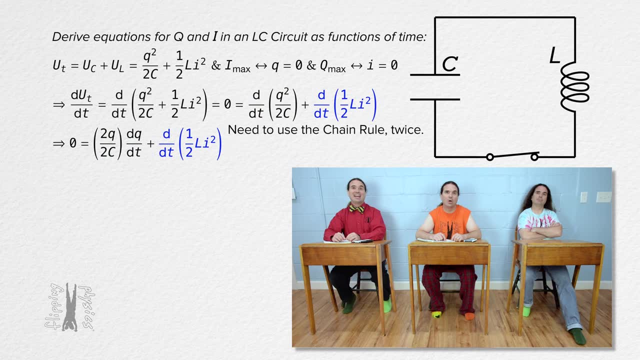 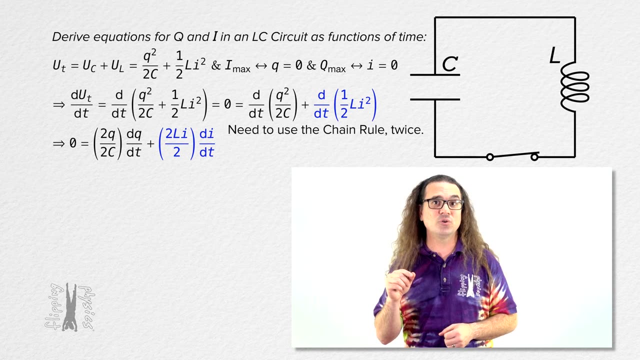 capacitance equals two times charge divided by two times capacitance, all times the derivative of charge with respect to time And the derivative with respect to time of one-half inductance times current squared equals two times inductance times current divided by two, all times the derivative. 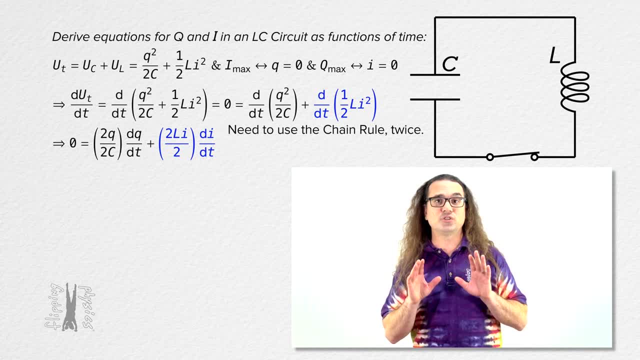 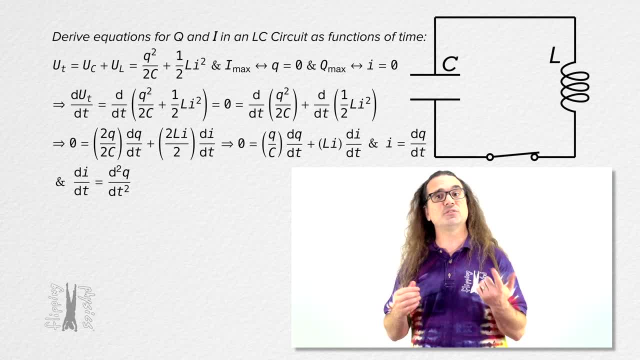 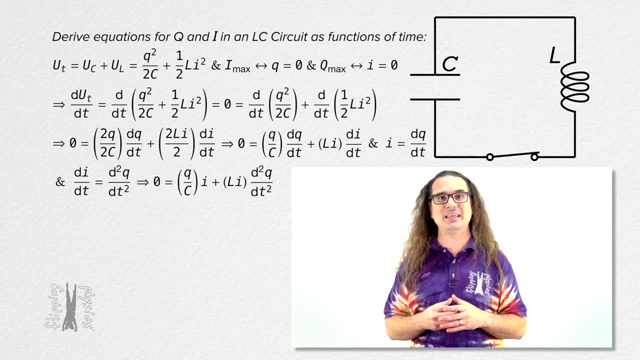 And the derivative of charge with respect to time. And the derivative of charge with respect to time And the derivative of current with respect to time equals the second derivative of charge with respect to time. Therefore, we can substitute current and the second derivative of charge with respect to time into our equation. Everybody brought current to the party. 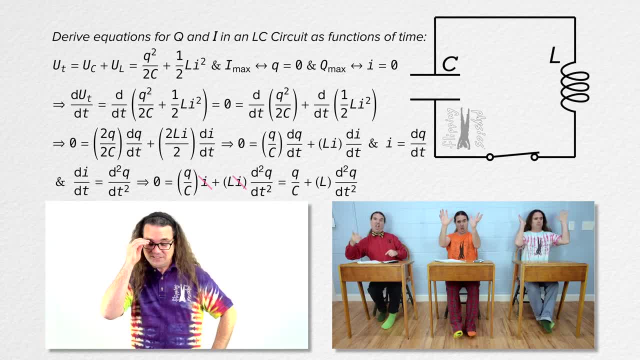 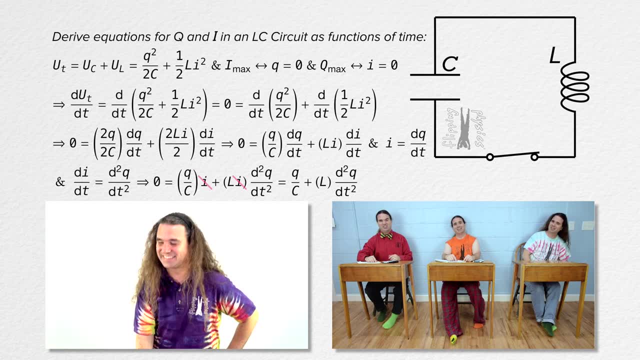 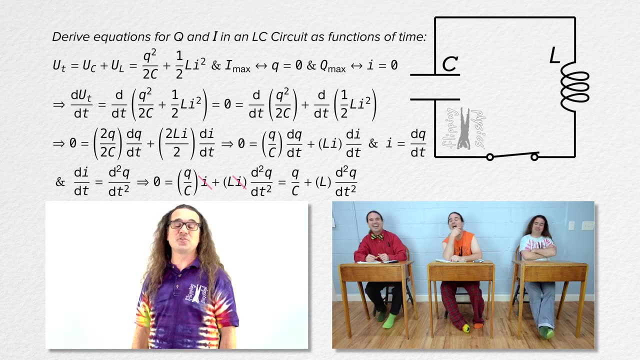 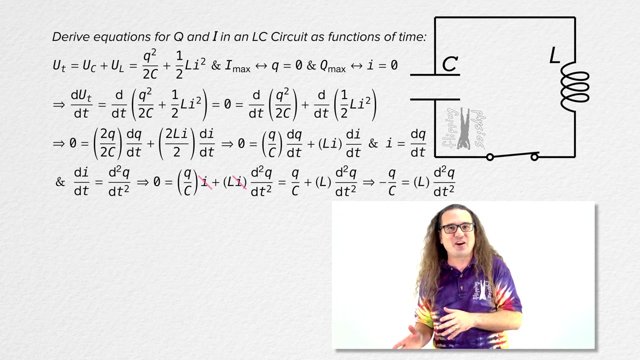 Everybody brought mass. Yeah, we can dance If we want to. We can leave your friends behind And your friends don't dance, And if they don't dance, they're no friends of mine. That was from dropping big air. We can move charge over capacitance to the other side and divide both sides by inductance. 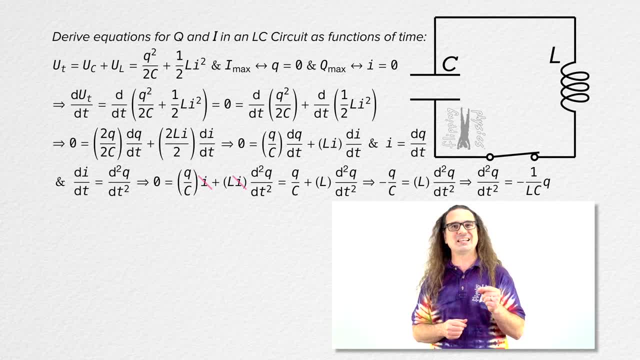 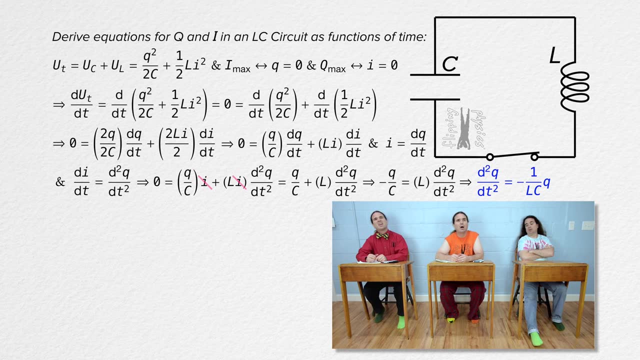 To get the second derivative of charge with respect to time equals the negative of the multiplicative inverse of inductance, times, capacitance, all times. Now, why would I arrange the equation this way? You remember it's simple harmonic motion, right Yeah? 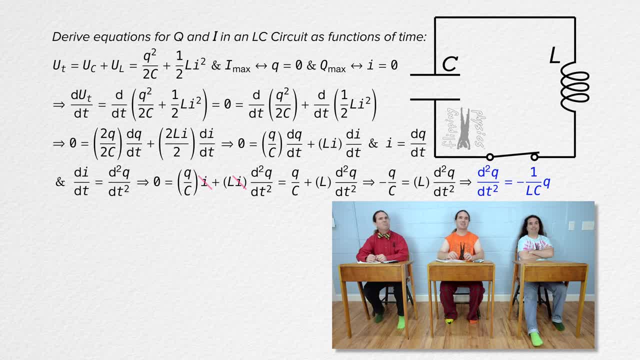 Oh, that's the equation definition for simple harmonic motion. It is, Yeah. The second derivative of a variable equals the negative of the square of angular frequency times the variable. Oh yeah, That means the square of angular frequency of an inductor-capacitor circuit. 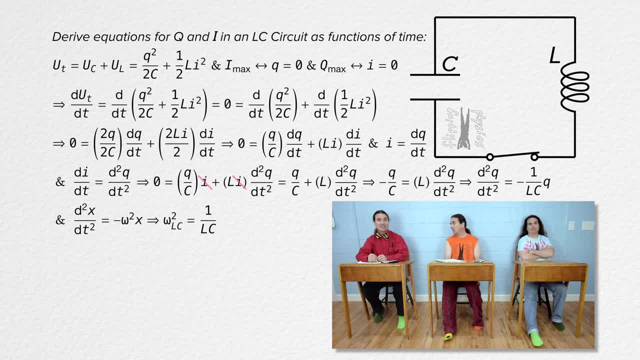 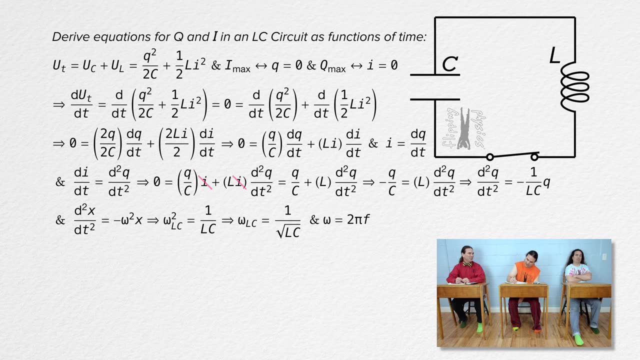 equals the multiplicative inverse of inductance times. capacitance Or the angular frequency of an inductor-capacitor circuit equals the multiplicative inverse of the square root of inductance times, capacitance. Right And angular frequency of simple harmonic motion equals 2 pi times frequency And frequency equals the multiplicative inverse of period. 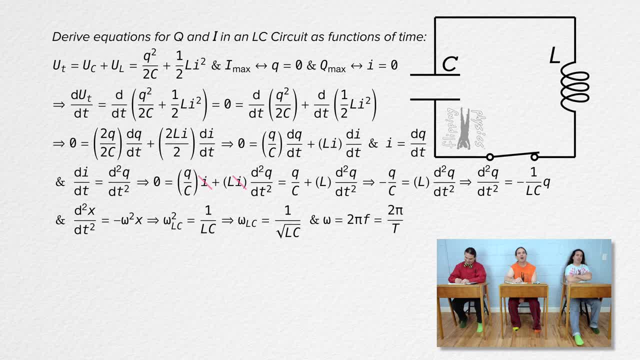 So angular frequency equals 2 pi over period. That means period equals 2 pi over angular frequency. And the angular frequency of an LC circuit equals 2 pi over the multiplicative inverse of the square root of inductance times capacitance, Or 2 pi times the square 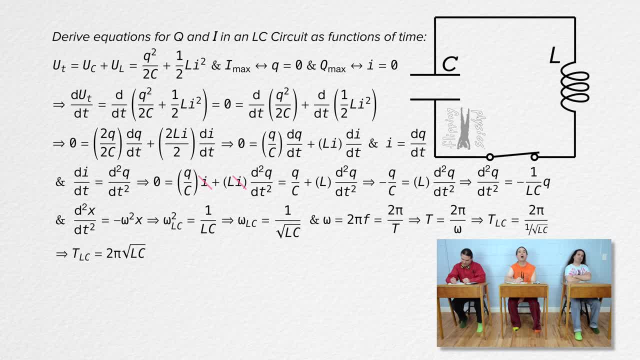 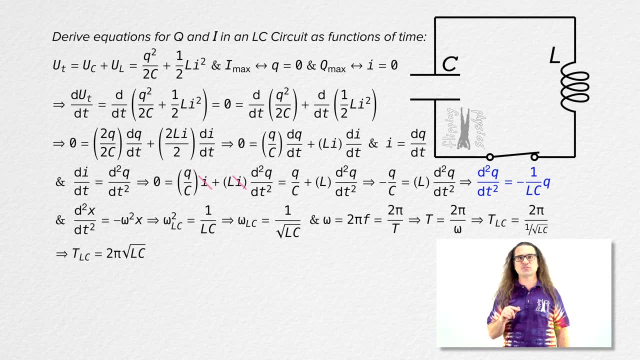 root of inductance times: capacitance. Well done everybody. So far we have proven an LC circuit is in simple harmonic motion And we have derived equations for its angular frequency and period. Recall that an equation which fits the equation definition for simple harmonic motion, Bobby. 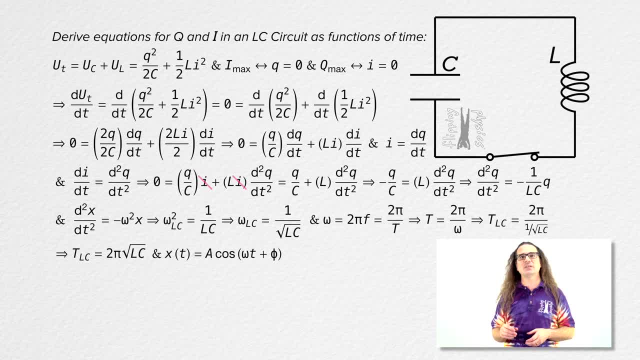 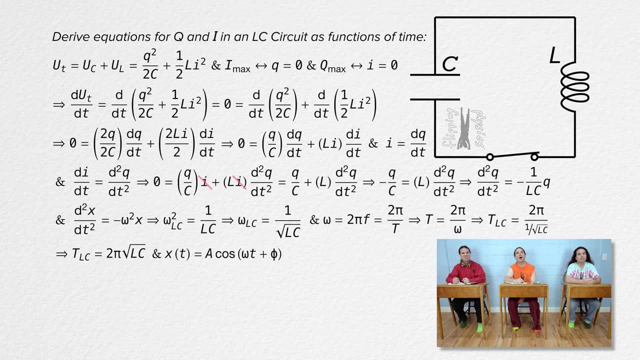 mentioned is …. x as a function of time equals amplitude times the cosine of the quantity. angular frequency times time plus phi, the phase constant. Billy, what is the equivalent equation for this inductor-capacitor circuit? Well, instead of x in our simple harmonic motion equation, we have charge on the capacitor. 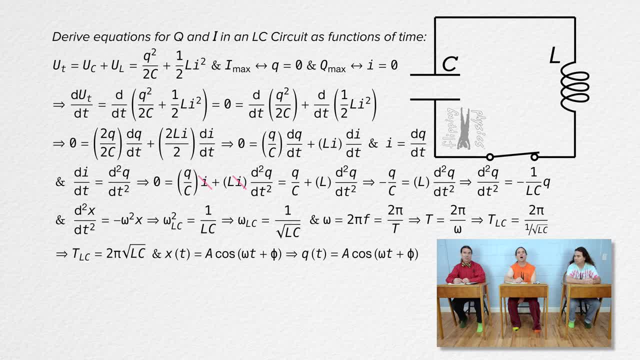 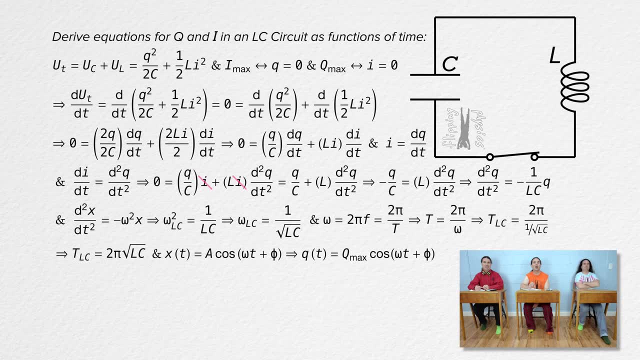 So charge on the capacitor, as a function of time, equals amplitude. However, for charge, the amplitude equals the maximum charge. So maximum charge times cosine of the quantity …. angular frequency times, time plus phase constant. However, angular frequency equals the multiplicative inverse of the square root of inductance times capacitance. And for this inductor, 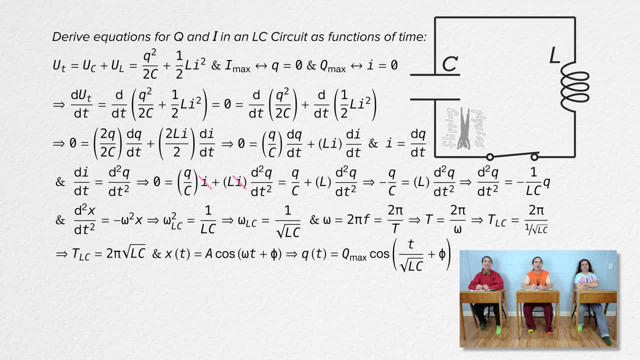 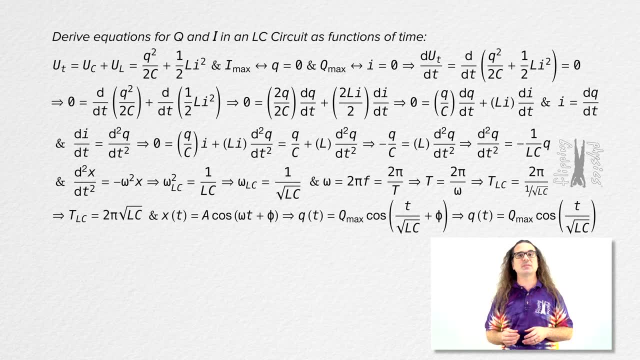 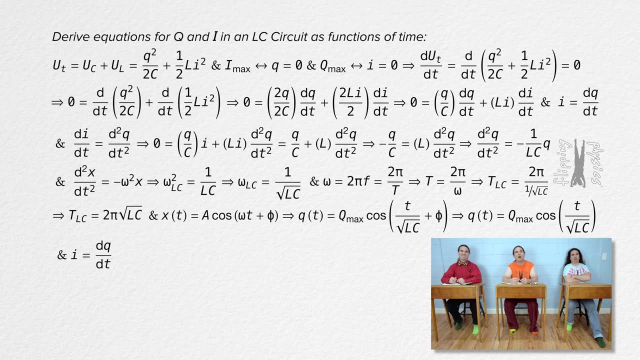 capacitor circuit. the initial charge on the capacitor is at its maximum value, which means the phase constant has to be zero. Thank you, Billy Bo. please determine the current through the inductor as a function of time. Sure Current equals the derivative of charge with respect to the current. 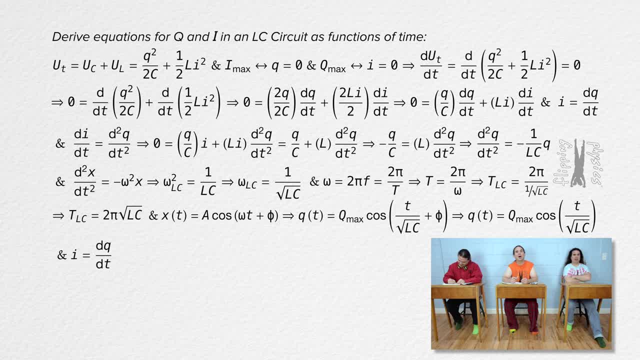 So we just take the derivative, with respect to time, of the equation for charge on the capacitor. Billy just derived The derivative of that equation …. we have to use the chain rule, So current, through the inductor with respect to time equals …. the derivative of cosine is negative, sine. 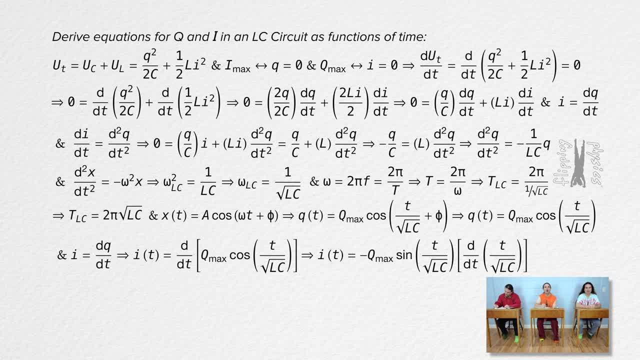 So negative charge: maximum times the sine of time over the square root of inductance times capacitance, all multiplied by the derivative with respect to time. Please go ahead, Billy. …. the derivative with respect to time of time over the square root of inductance times capacitance. 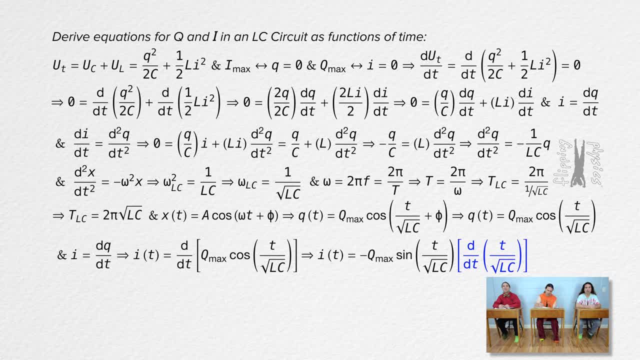 … and the derivative with respect to time of time over the square root of inductance times capacitance is …. or a tacticец …. the multiplicative inverse of the square root of inductance times capacitance …. …and the maximum value for sine of anything is 1.. 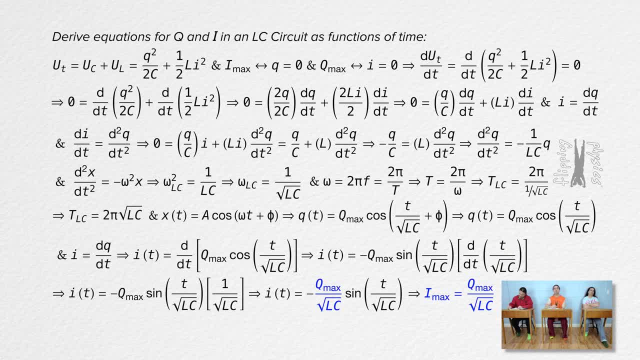 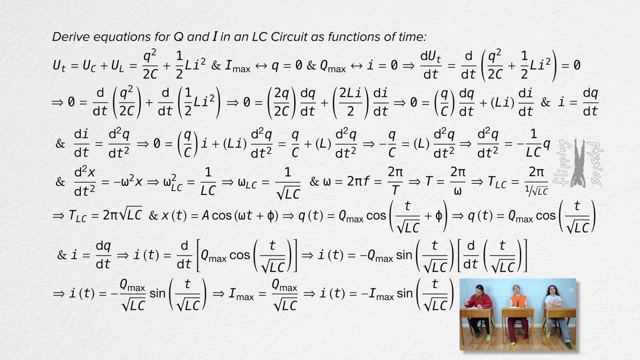 That means the maximum value for current through the inductor equals charge maximum over the of inductance times capacitance. So current through the inductor as a function of time equals the negative of maximum current times, the sine of the quantity time over the square root of inductance times capacitance. 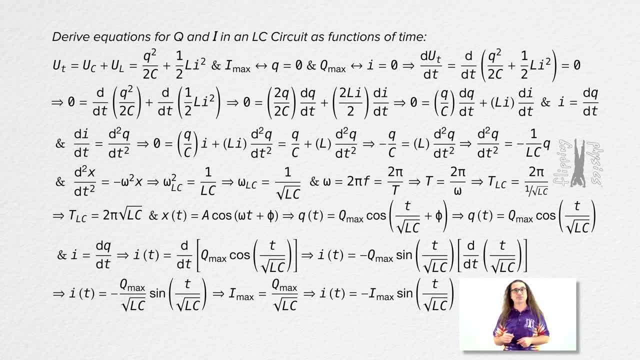 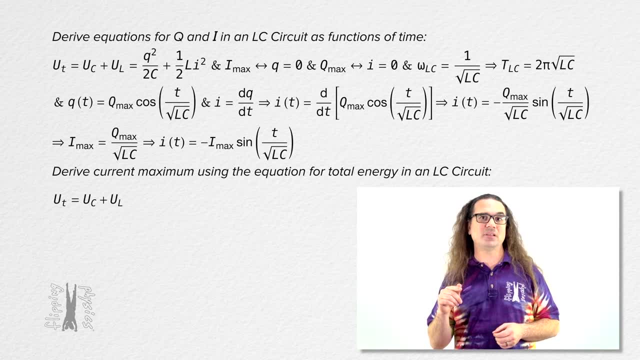 Valid point, Bobby, And we can also determine that equation for maximum current using the energy equations. The total energy in the LC circuit equals the energy in the capacitor plus the energy in the inductor. That equals charge squared over 2 times capacitance plus one-half inductance. 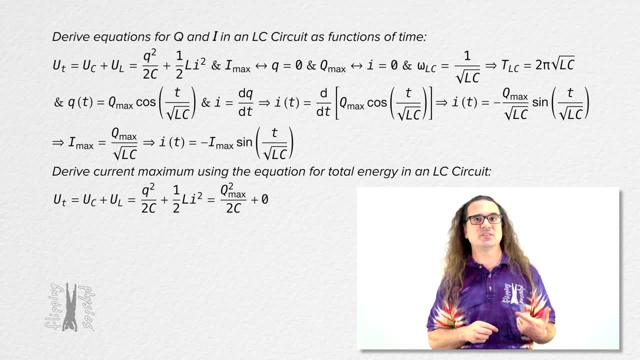 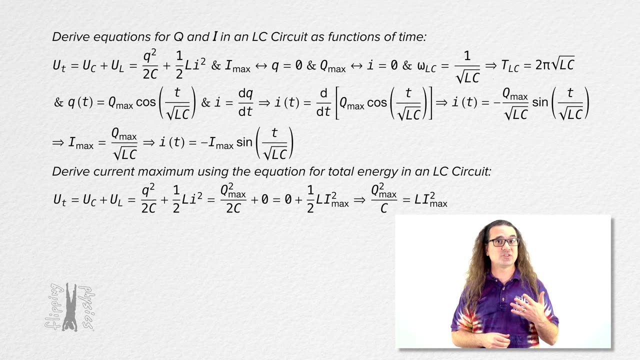 times current squared. When there is zero energy in the inductor, all the energy is in the capacitor and the charge is at a maximum. And when there is zero energy in the capacitor, all the energy is in the inductor and the current is at a maximum. One-half cancels out. We can solve for. 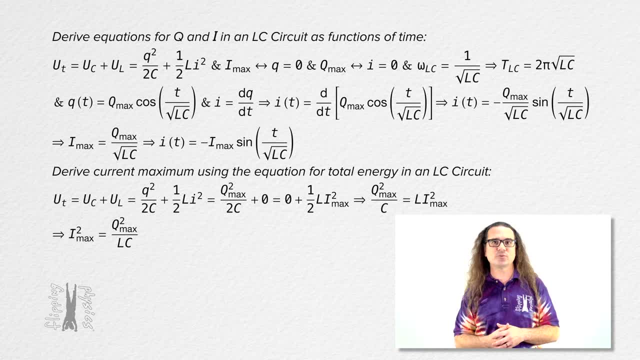 current maximum squared, And taking the square root gives us the same equation you just derived, Bobby. The maximum current through the inductor equals the maximum charge on the capacitor divided by the square root of the capacitor, times the charge squared over 2 times the energy in the 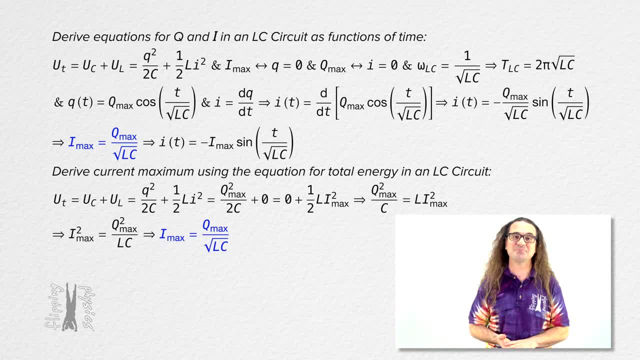 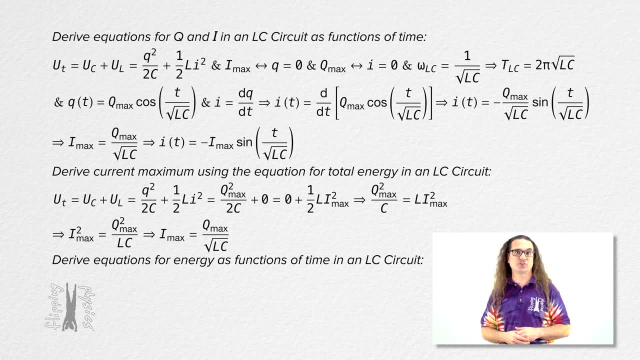 capacitor plus the square root of inductance, times capacitance. Cool, Nice Yeah. Now we can also determine equations for energy as functions of time in this inductor capacitor circuit. Billy, please determine that for the capacitor, Bobby, for the inductor. 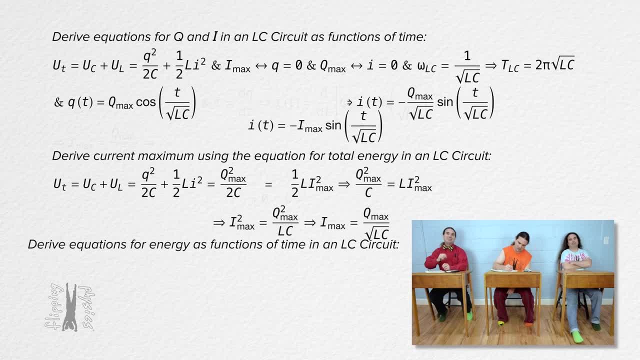 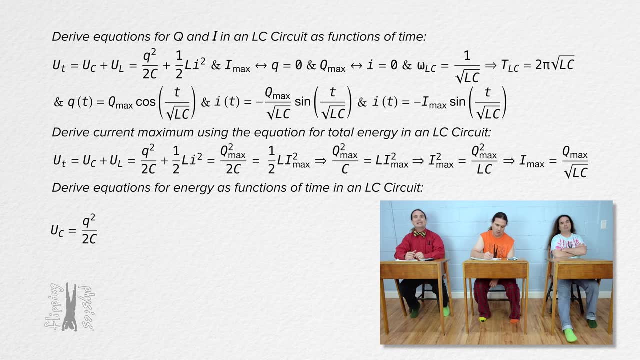 and Bo for the total LC circuit. Absolutely, The energy stored in the electric field of the capacitor equals charge squared divided by 2 times capacitance. That means the energy stored in the electric field of the capacitor is a function of time, equals the square of the quantity charge maximum times cosine of the quantity. 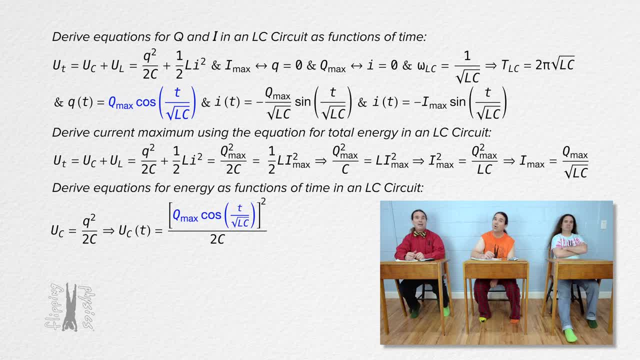 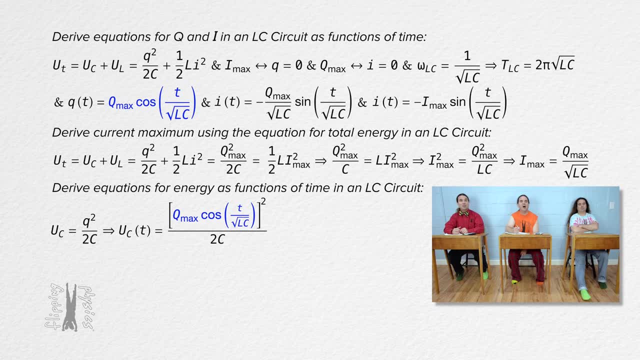 time divided by the square root of inductance times capacitance. all divided by 2 times capacitance, That means the energy stored in the electric field of the capacitor is a function of time. equals charge maximum squared divided by 2 times capacitance. times cosine squared of the quantity. 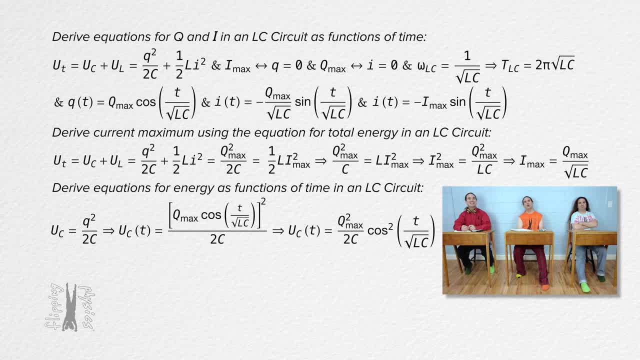 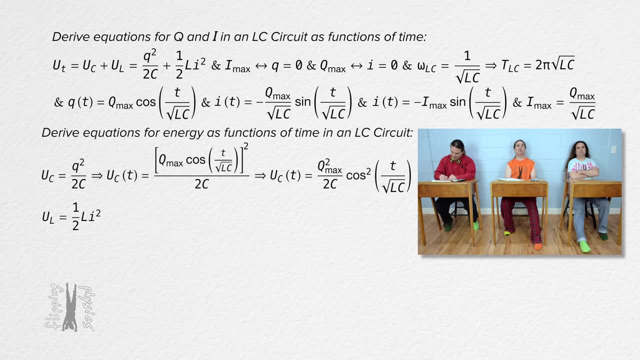 time divided by the square root of inductance times. capacitance, The energy stored in the magnetic field of an inductor equals one-half inductance times. current squared. That means the energy in the inductor as a function of time equals one-half inductance times the square of the. 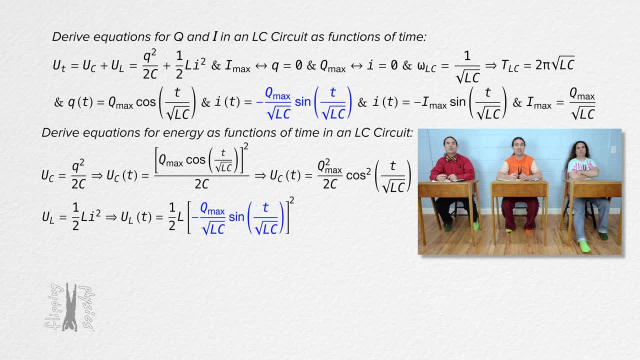 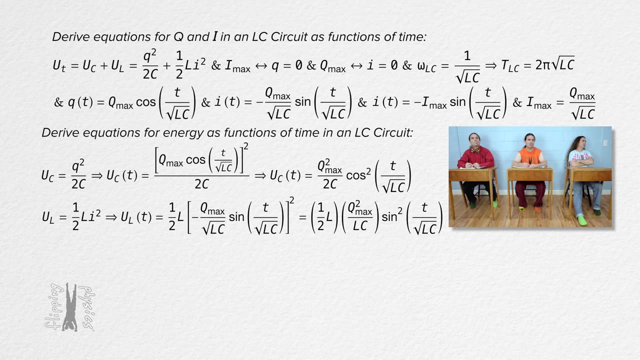 quantity negative charge maximum over the square root of inductance times capacitance: all times the sine of the quantity time over the square root of inductance times capacitance. That equals well negative. 1 squared is just 1, so one-half inductance times charge maximum squared over. 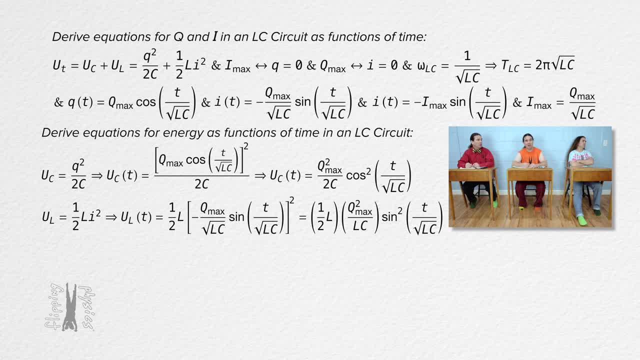 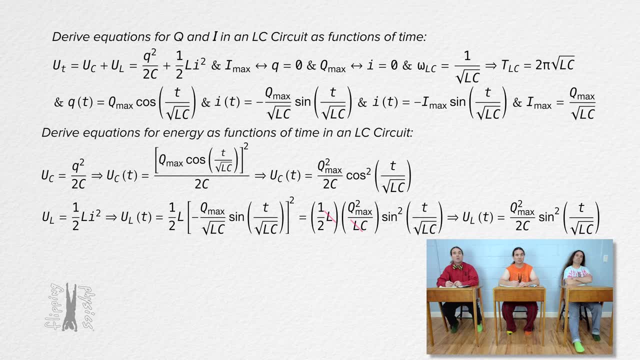 inductance times capacitance all times sine squared of time over the square root of inductance times capacitance. Inductance cancels out and we get that the energy stored in the magnetic field of the inductor as a function of time equals charge maximum squared over 2 times capacitance. 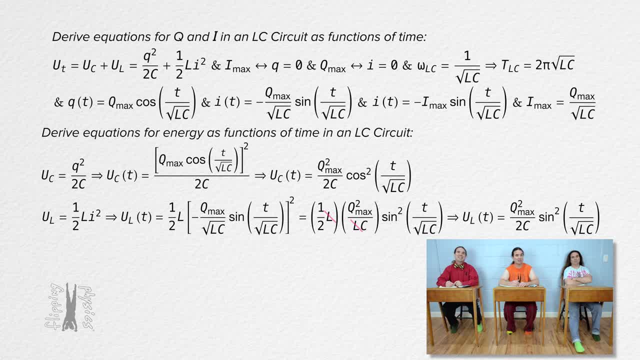 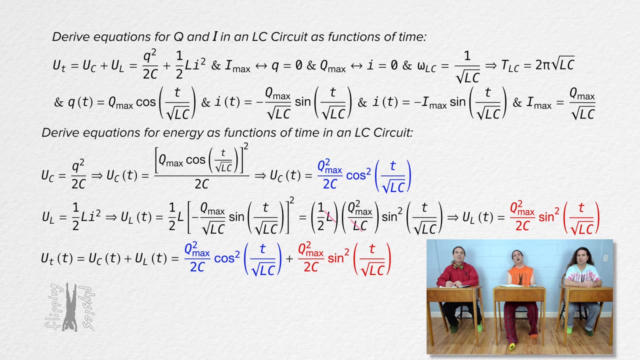 times sine squared of time over the square root of inductance, times, capacitance And Bo the total energy in the LC circuit as a function of time. please Don't we just sum the two equations Billy and Bobby just derived. Yes, but what can we do with that equation? 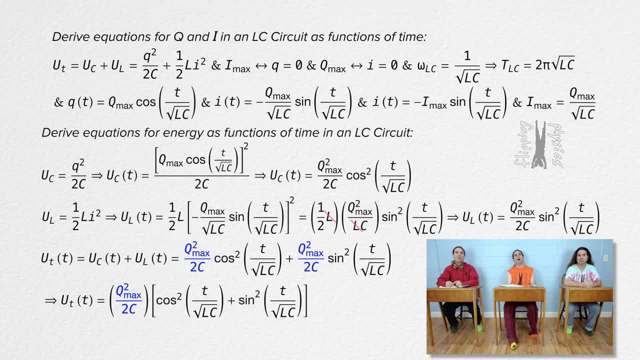 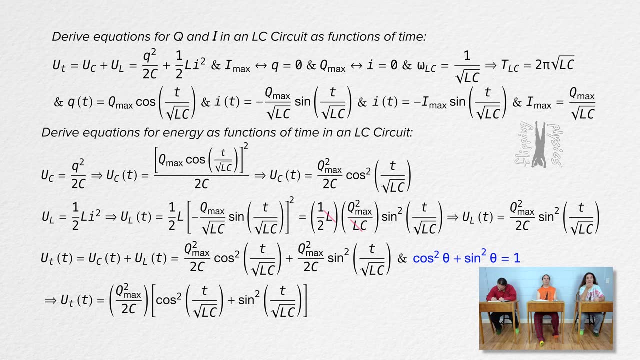 Uh, we can factor out maximum charge squared over 2 times capacitance. That's about it. Oh No, I see it. So okay. okay, Cosine squared theta plus sine squared theta equals 1, so that whole bracketed expression equals 1.. That means the total. 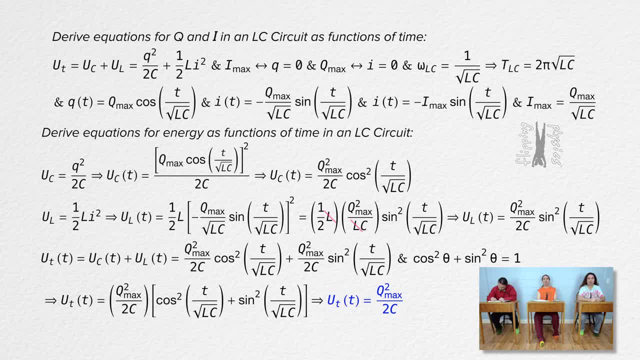 energy in the LC circuit as a function of time equals maximum charge squared over 2 times capacitance. And that actually does not change over time, because the total energy in the LC circuit is constant, because all the wires are ideal and have zero resistance, so no energy. 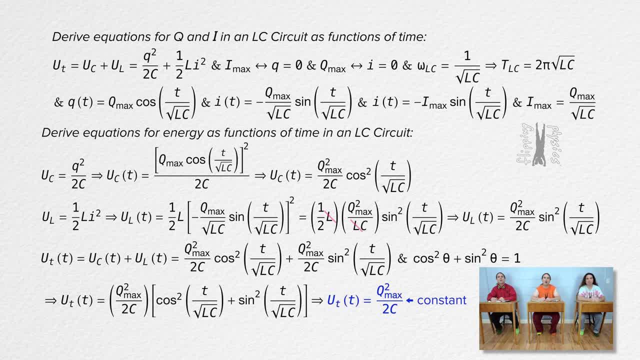 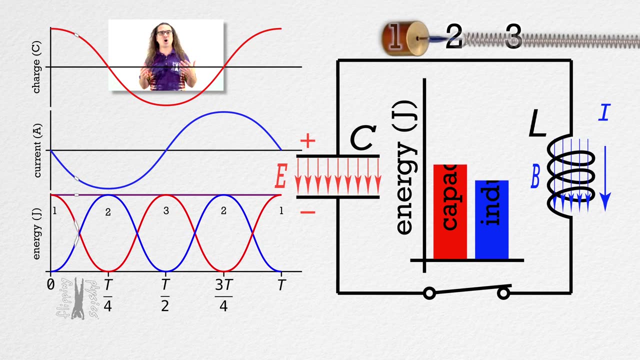 is being dissipated in the circuit. We just proved that Exactly, Bo thanks. Now we have derived all these equations for the inductor capacitor circuit. however, we have yet to look at the graphs for the equations. So here is an animation showing all the graphs for all time-dependent equations we derived. 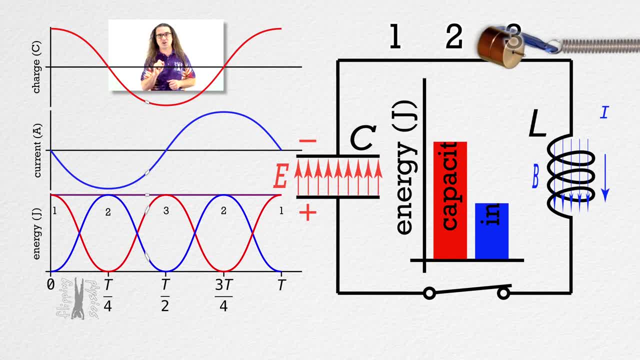 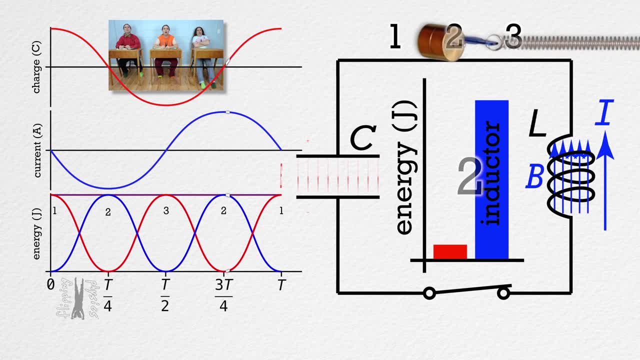 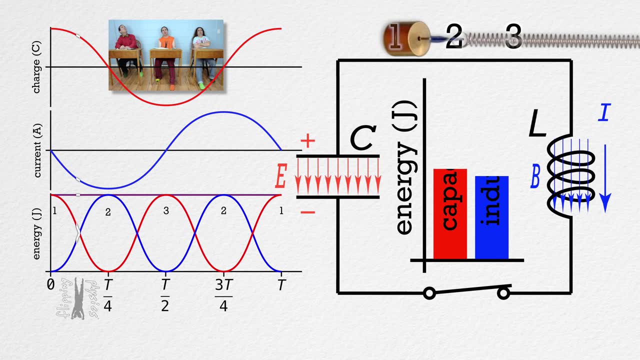 and how all the components of the LC circuit are changing. Oh, that is a lot. Yes, it is So I'll give you a moment to just take it in before we start talking about all the details. That's a lot. 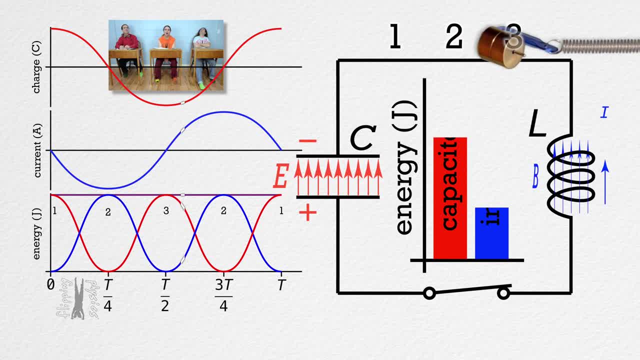 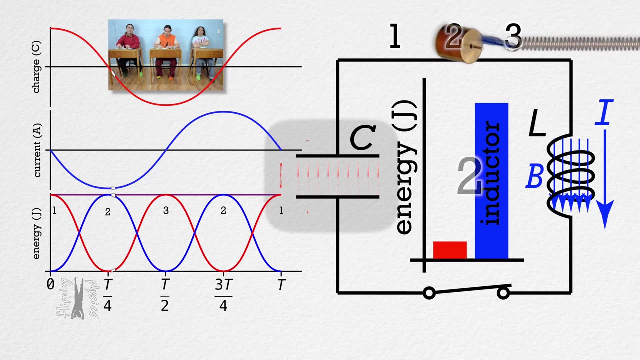 Here we go, Billy, looking at just the capacitor in the circuit. tell me what you see, Absolutely. When I look at the capacitor, I see that the capacitor has charges on the plates which increase and decrease over time and an electric field which increases and decreases over time. 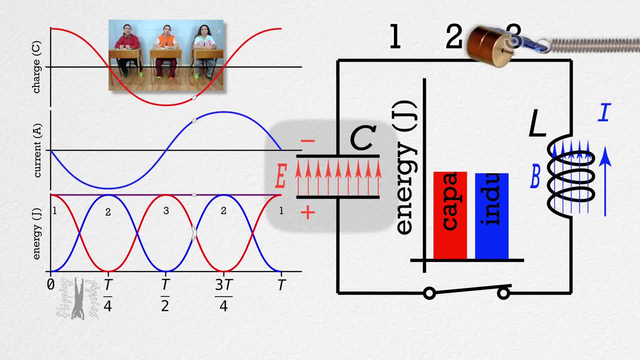 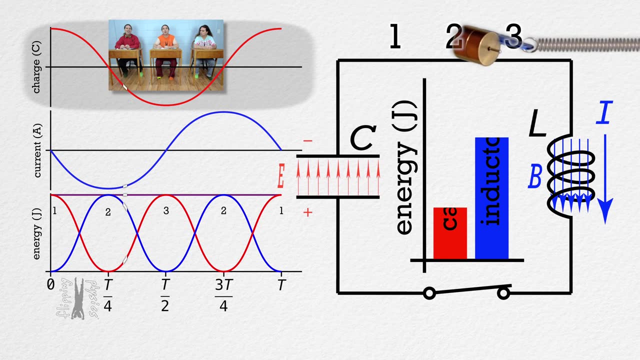 And the direction of the electric field switches and the locations of the positive and negative charges on the plates also switch When both of those are equal to zero. actually, you can see how the charge changes as a function of time on the graph. That is the red cosine curve. I like how you put that. 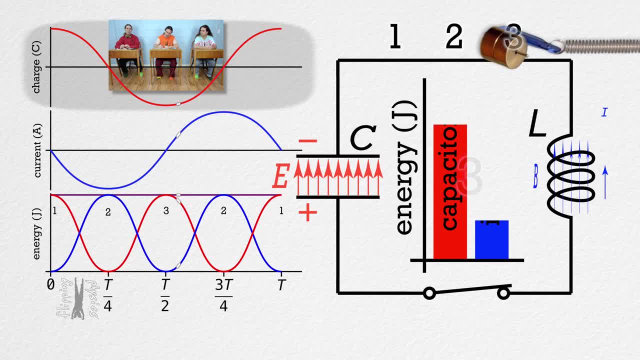 moving white part of the graph there so we can see where the charge is on the graph and compare that to what the charge is on the capacitor in the circuit. Thanks, You are welcome. Oh, and you can see the energy stored in the capacitor as well. 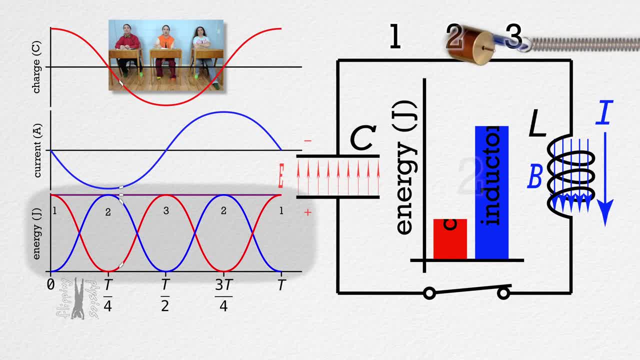 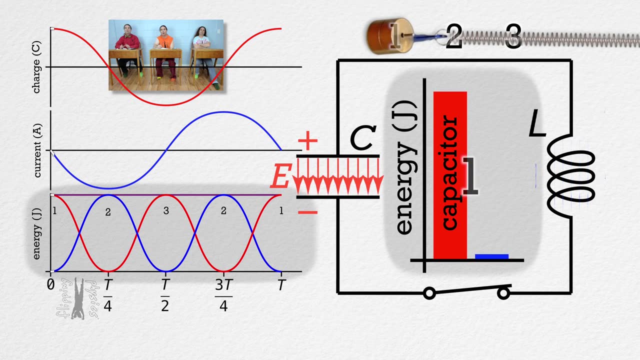 There is both an energy curve with respect to time and an energy bar graph. Both of those show the energy in the capacitor in red to match the red charge curve, the red charges on the capacitor and the red electric field in the capacitor. Again you can see how the energy in the capacitor changes as a function of time. in all of those, 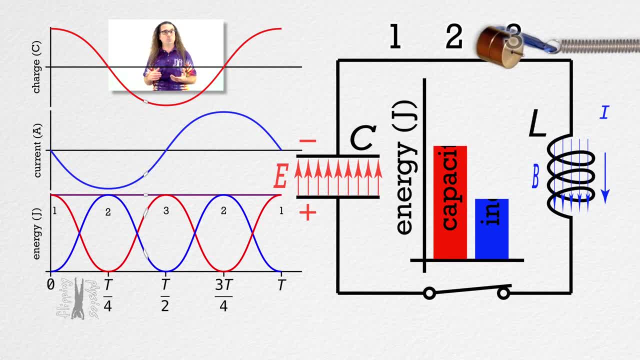 Very nice. Thank you, Billy Bo. what do you see when you look at just the inductor in the lc circuit? Sure, Looking at just the inductor… Well, the magnetic field in the inductor is the 69.7 van. 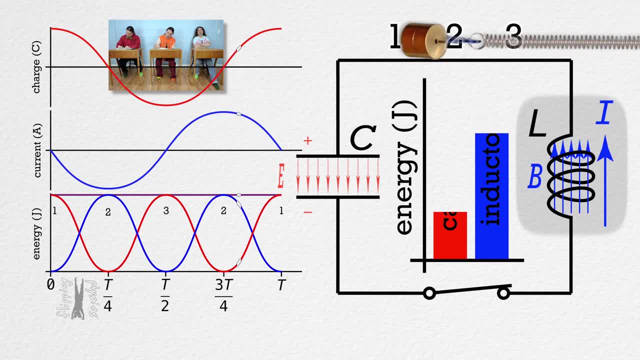 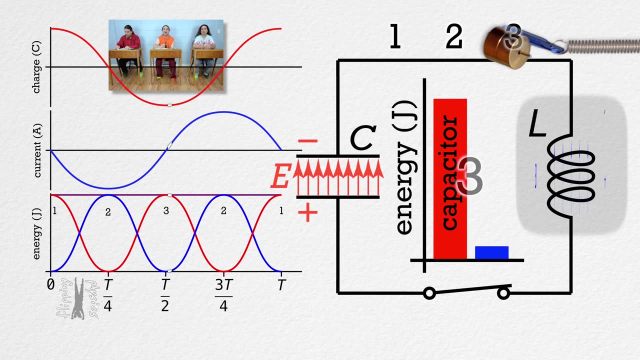 W. Looking at just the inductor, well, the magnetic field in the inductor is in blue and is increasing and decreasing and changing directions, just like the electric field. Only the magnetic field in the inductor is at a maximum when the electric field in the capacitor is zero and the magnetic 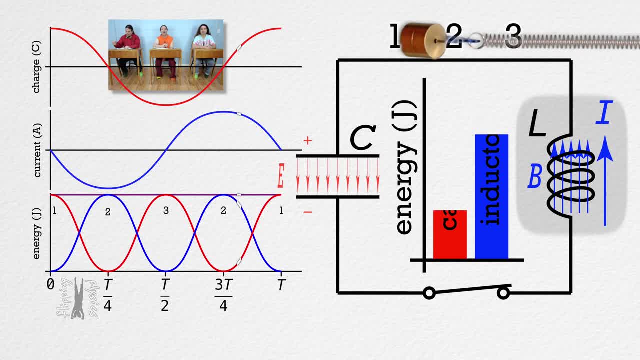 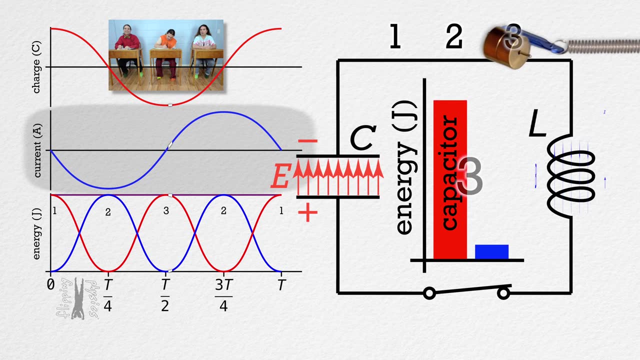 field in the inductor is zero when the electric field of the capacitor is at a maximum. The current, also in blue, through the inductor increases and decreases and changes directions, just like the magnetic field. There is also a blue current graph with the same white part to. 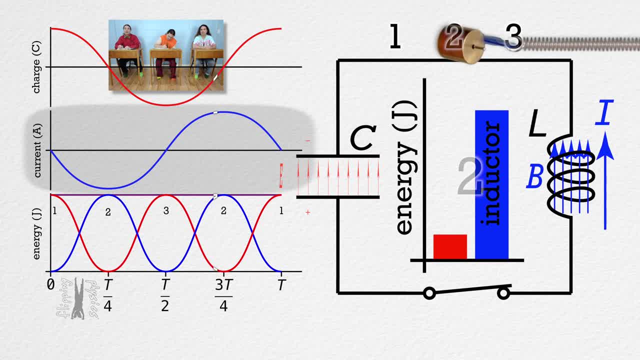 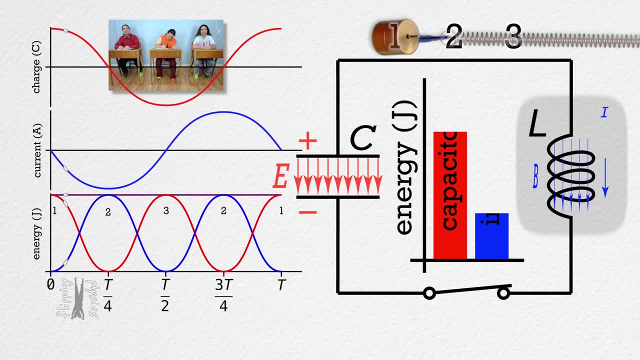 show what the current is at each moment in time in the LC circuit. Going back to the blue magnetic field in the inductor, we can see that it increases and decreases with the energy in the inductor, which is shown both in the blue energy bar graph for the inductor and the blue 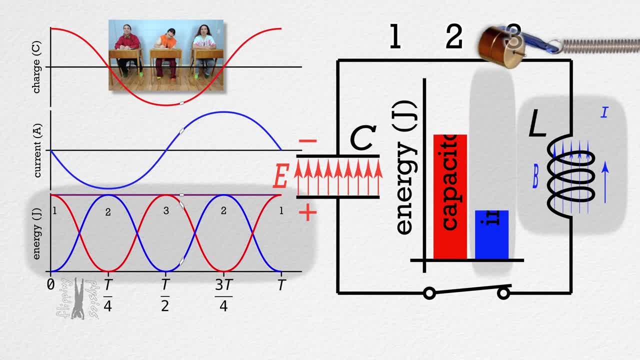 energy curve for the inductor. Oh, and that purple horizontal line on the energy as a function of time graph. that line must represent the total energy in the LC circuit. Yeah, Blue and red make purple. Nice one, Mr Pete. 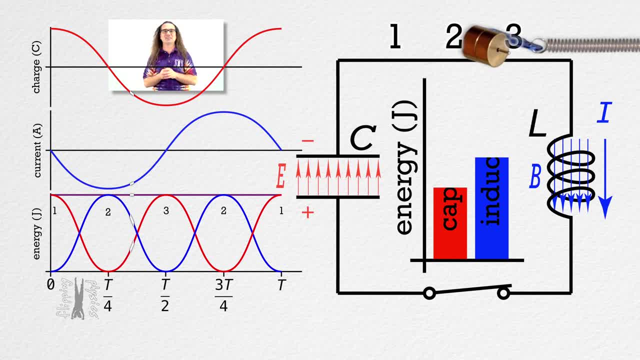 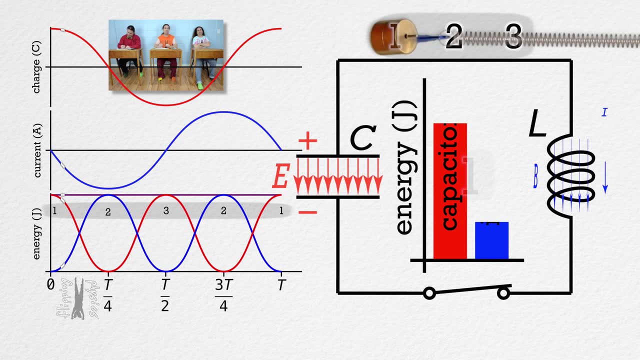 Sure, Nice. Thanks, Glad you appreciate it, Bobby. nobody has talked about the numbers or the mass spring system. Please discuss what those are. Okay, All the numbers show the locations in simple harmonics where the energy is at a maximum and at a minimum, For example at position 1,. 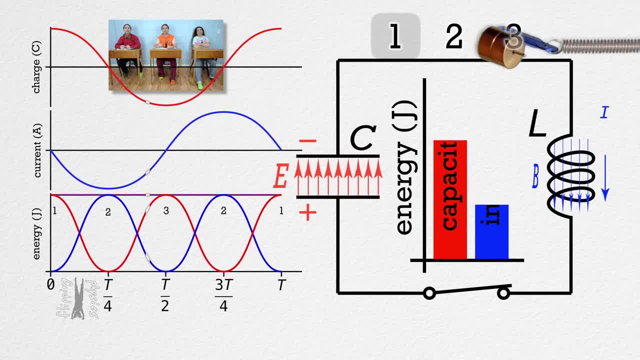 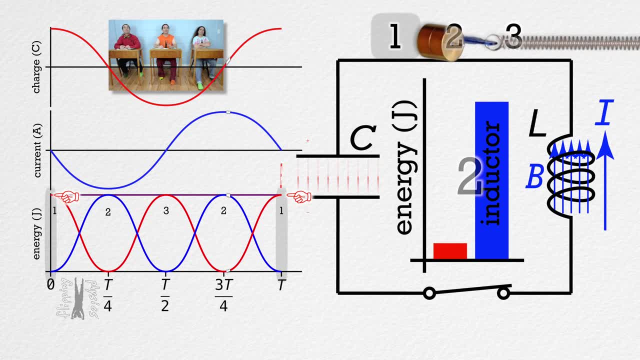 the horizontal mass spring system has its maximum elastic potential energy and zero kinetic energy. Also at position 1,. the LC circuit has its maximum energy in the electric field of the capacitor and zero energy in the inductor because there is no current through and no magnetic field in. 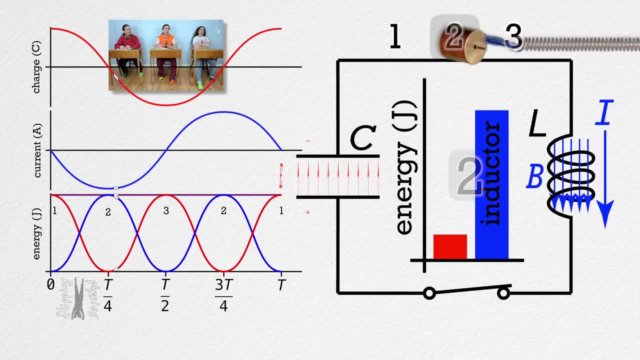 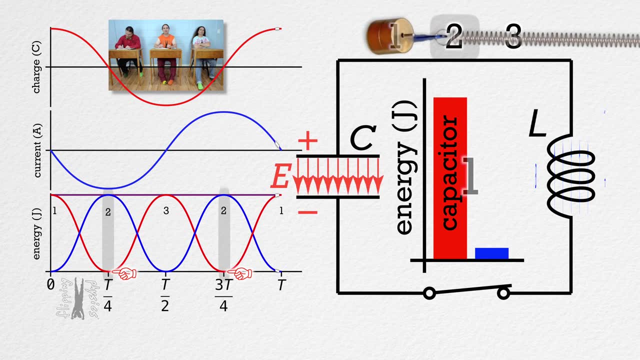 the inductor. At position 2, the horizontal mass spring system is at the equilibrium position, so it has zero elastic potential energy and its maximum kinetic energy Also at position 2,. the LC circuit has zero electric field in the capacitor and zero energy in the capacitor. 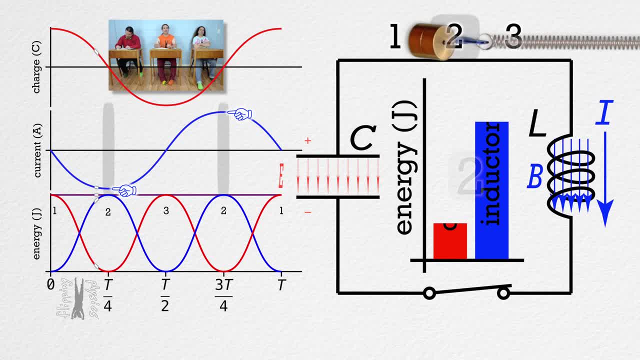 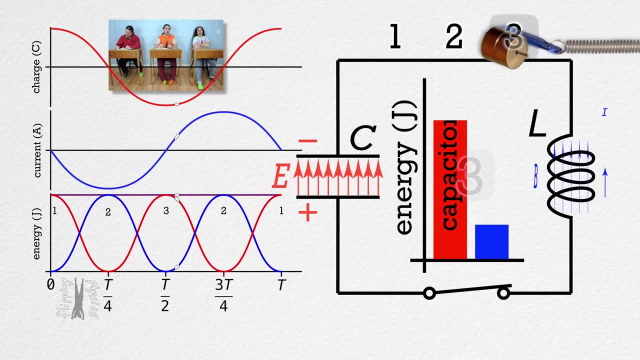 and its maximum magnitude current through the inductor, maximum magnitude magnetic field in the inductor and maximum energy in the inductor. At position 3, the horizontal mass spring system has the same energy values as it had has at position 1,. however, the mass is on the opposite. 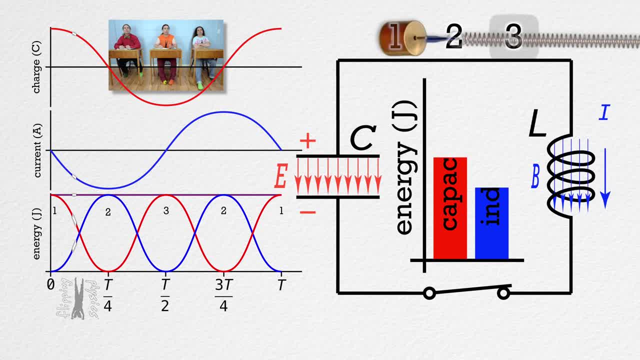 side of the equilibrium position. The same is true at position 3 for the LC circuit. The energy values for the LC circuit at position 3 are the same as at position 1,, however, the charges on the plates have switched and the direction of the electric field is reversed. 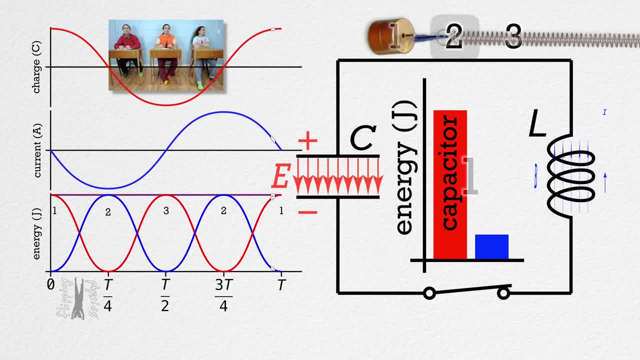 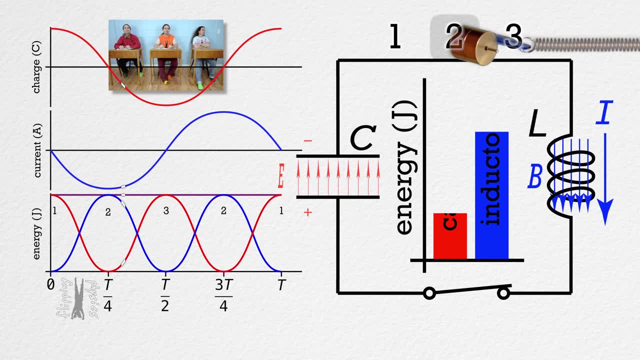 And then back at position 2,. the horizontal mass spring system has the same energy values as the last time it was at position 2, only the direction of the velocity of the mass is reversed. This is just like the position 2 for the LC circuit. All the energy values are the same. 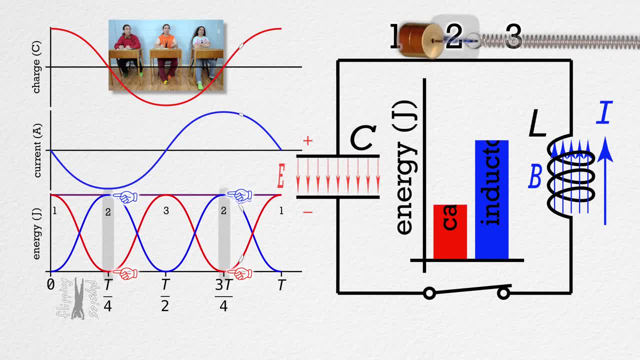 as the last time it was at position 2, only the direction of both the current and magnetic field are reversed from the last time the LC circuit was at position 2.. This LC circuit really is in simple harmonic motion, just like a horizontal mass spring system. 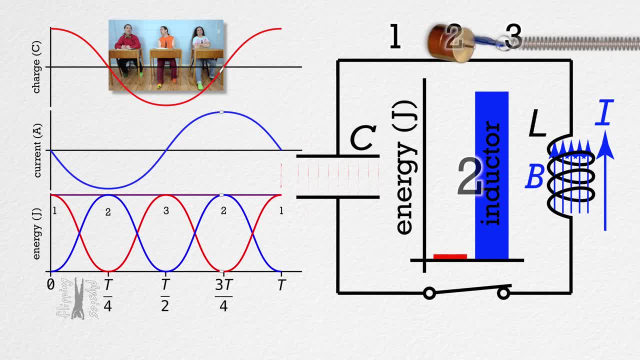 Actually, we should talk about the period as well. From position 1 to bottom of the equation, we can see that the current and magnetic field are reversed. From position 1 to bottom of the equation, we can see that the current and magnetic field are reversed. 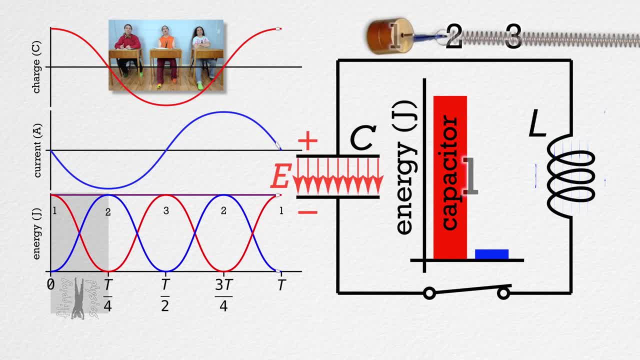 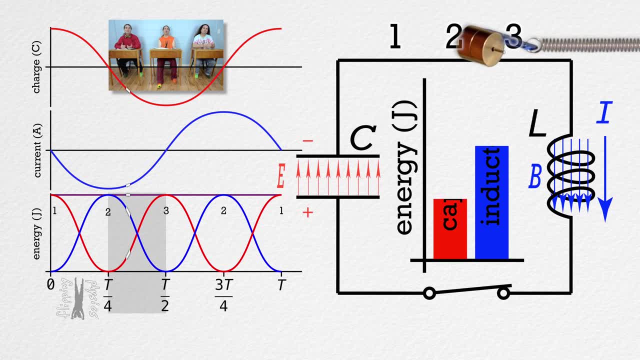 Position 2 is one-fourth of a full cycle, so the time it takes is one-fourth of the period. And well, that's true between every position. It takes one-fourth of the period between every position. Yeah, But why is the current negative when the charge is positive? 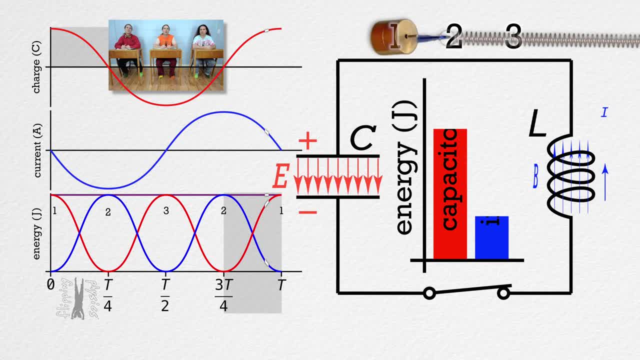 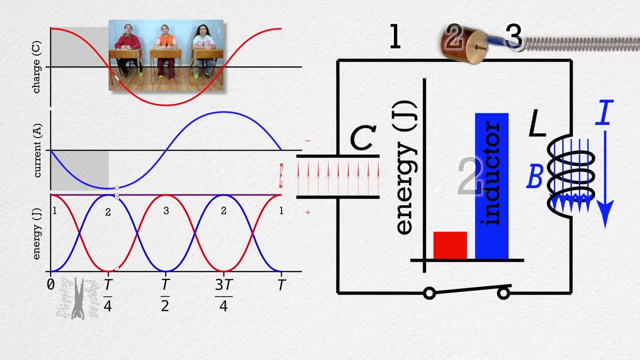 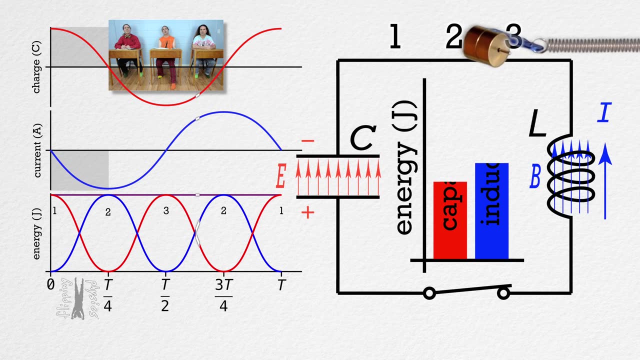 What do you mean? Look at the charge and current as function of time graphs. During the first quarter of a period, the charge on the capacitor is positive, yet the current is negative. That seems weird. Yeah, sure, I can see how that would seem strange at first. However, it really isn't. It just comes. 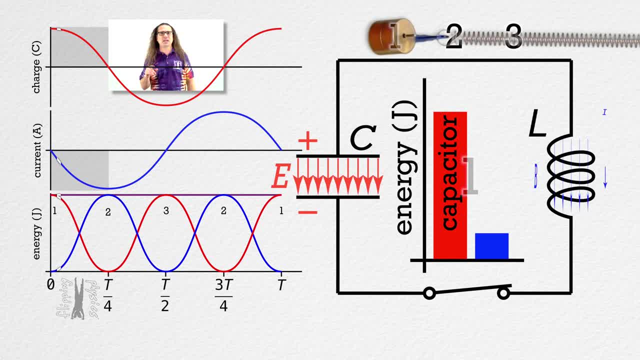 down to which plate's charge we are graphing and which direction we define for positive current. In this example, I have defined the charge we are graphing as the charge on the top plate. If we instead graphed the charge on the bottom plate, the curve would be flipped over the horizontal time. 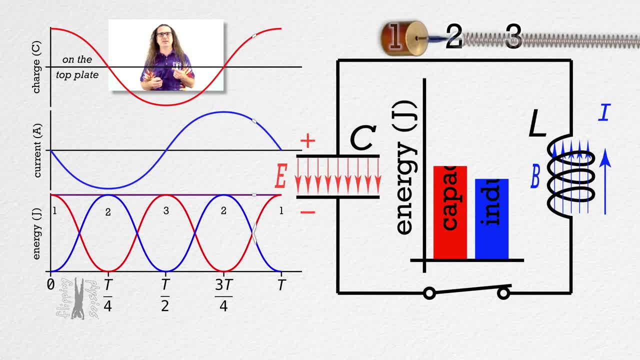 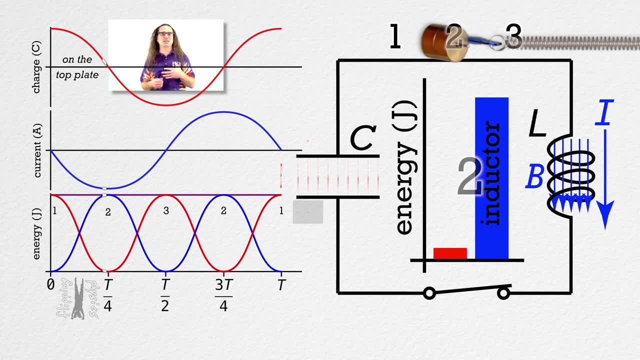 axis, You could see that the charge on the top plate would be flipped over the horizontal time axis because the charge on the bottom plate starts out at position 1 as negative. Again, if we were graphing the charge on the bottom plate, it would be negative at position 1 and positive at. 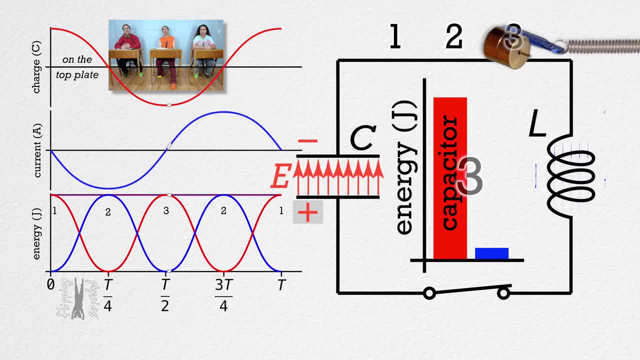 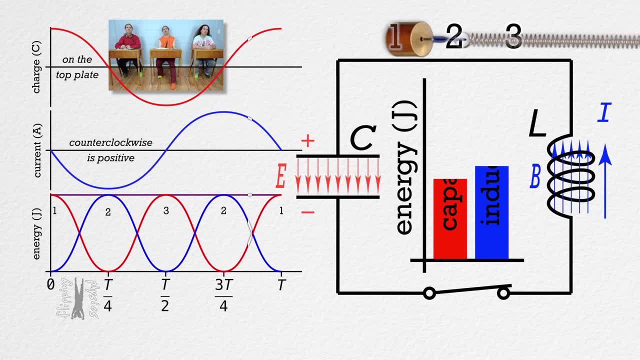 position 3.. Okay, That makes sense, And you must have defined positive current as being in the counterclockwise direction. At the second position 2,, the current is positive and counterclockwise. If you had defined the clockwise direction as being positive, the current is: 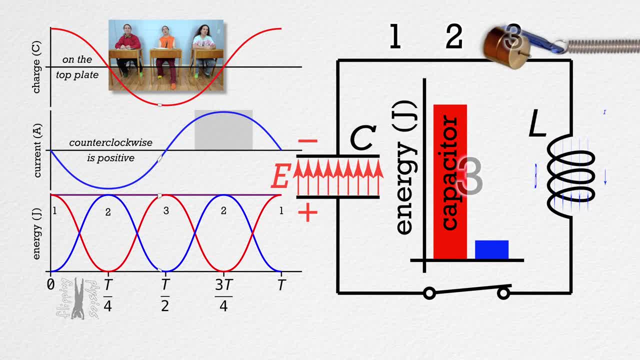 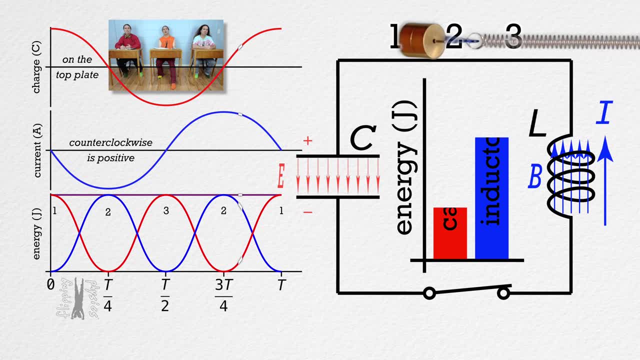 a function of time curve, who would also be flipped over the horizontal time axis. So it really just comes down to which capacitor plate you are graphing the charge as a function of time of, and which direction you define as positive for current through the inductor. 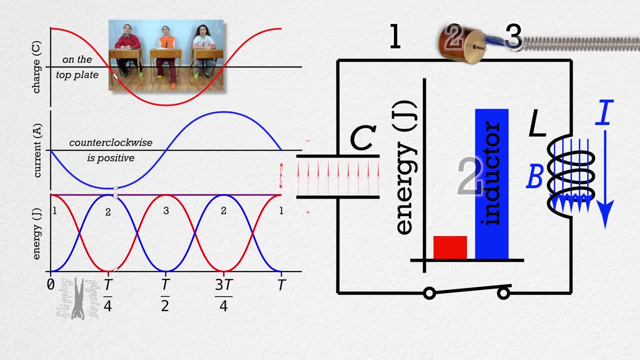 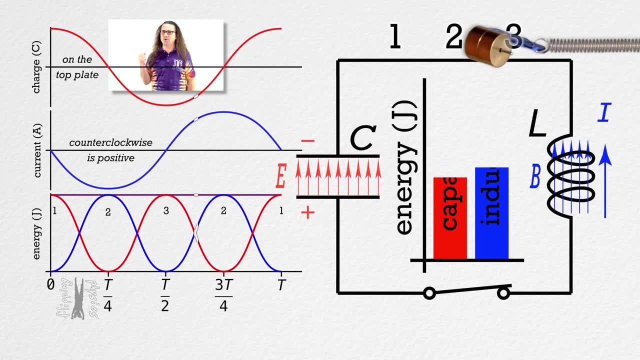 Yeah, That does make sense. Thanks, Mr P and Billy. You are welcome. Hold up, Mr P. I have another question. Yes, Bo, At position 2, how can the inductor have a positive current through the inductor? How can the inductor 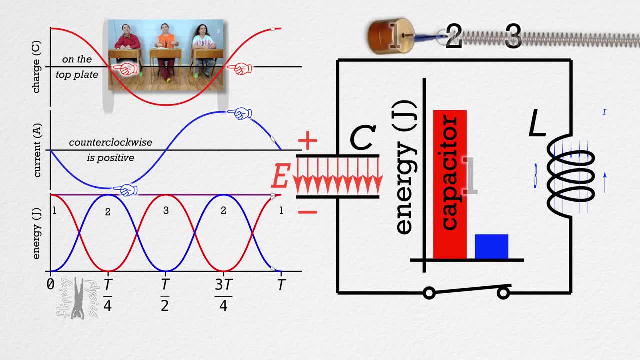 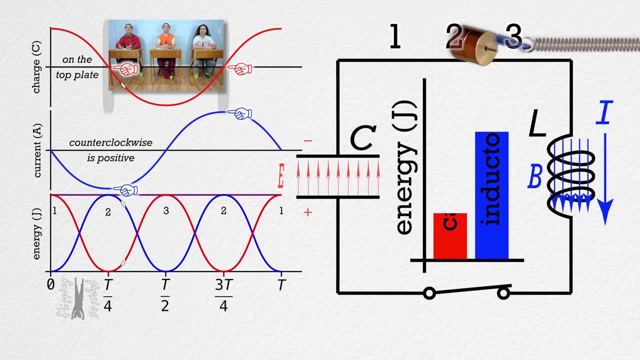 have current passing through it when there is zero electric potential difference across the capacitor? Oh yeah, Electric potential difference is what causes current, right? So how can current be flowing when there is zero electric potential difference in the circuit? Bobby, do you have something to say? 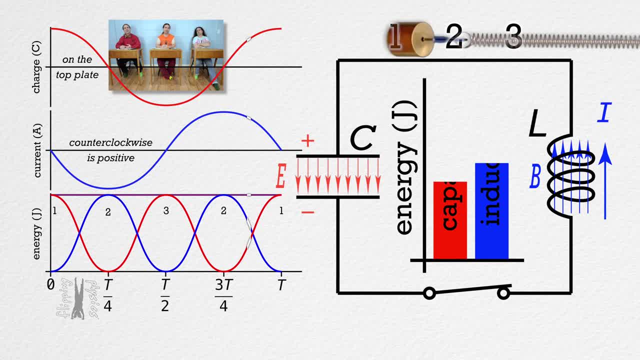 Well, take a moment to look at the horizontal mass spring system as it passes through position 2.. If we ask the same question of the horizontal mass spring system, it would be: how can the mass, the mass, still be moving at position 2 when there is no restoring force accelerating the mass, correct? 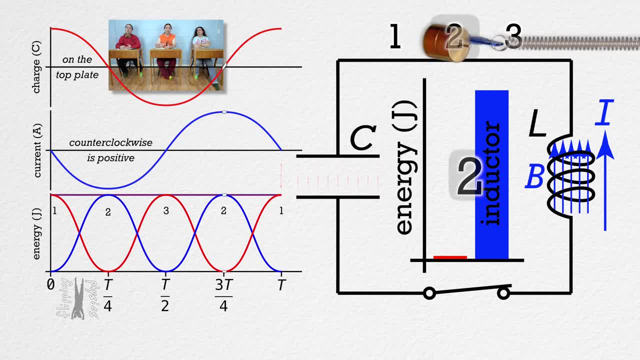 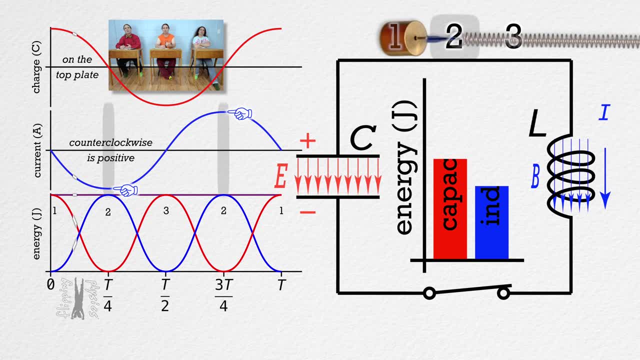 Sure, The mass still has velocity at position 2.. In fact, it has its maximum magnitude velocity at position 2, just like the LC circuit has its maximum magnitude current at position 2.. The mass is simply experiencing zero change in its velocity at position 2 because its acceleration. 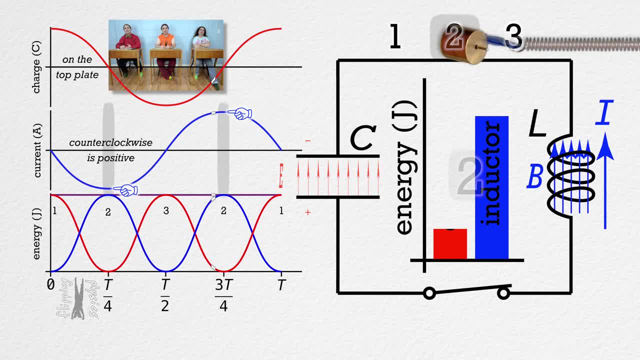 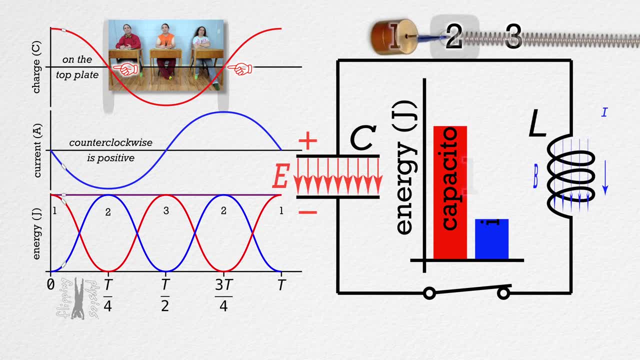 at position 2 is zero, just like the current in the LC circuit is not changing at position 2.. So the mass keeps its momentum at position 2 because there is zero electric potential difference across the capacitor. The inertia of the mass in the horizontal mass spring system keeps the mass.